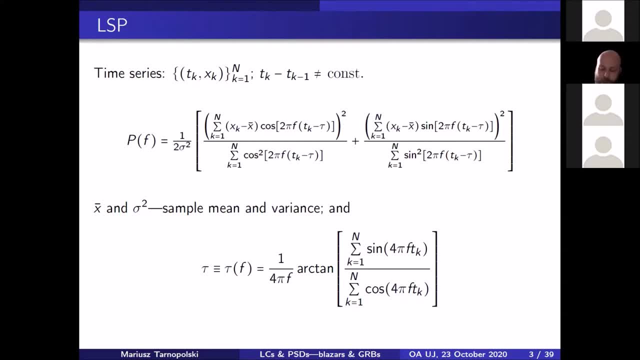 choices of the frequencies corresponding to the length of the data and the Nyquist frequency will be used. The number of frequencies is chosen to deliberately oversample the periodogram to constrain the shapes of the peaks accurately. They usually go from thousands to thousands to tens of thousands. This is an advantage over the usual common Fourier spectrum, since 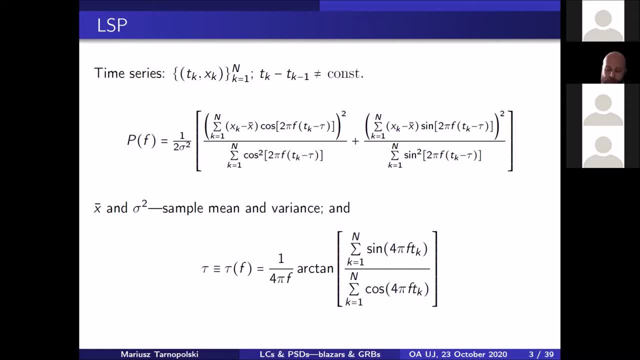 in the Fourier case, the number of frequencies is limited and precisely governed by the data, And with the LSP we have more freedom And basically the LSP is based on an assumption that the examined signal can be decomposed into sinusoidal components. For simplifying, it's a fancy. Fourier: 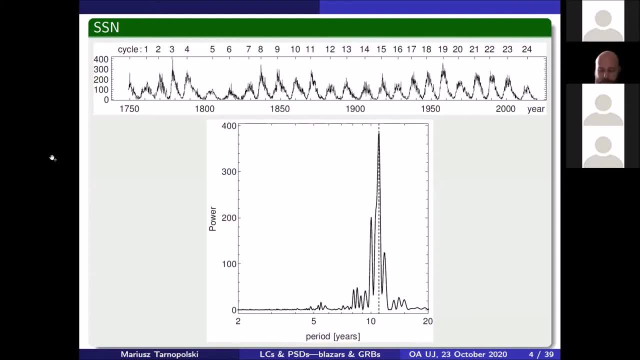 So, as an example, let's take the sequence of the Sun-Squat numbers, which has this well-known 11-year cycle, And indeed in the LSP you can see some peaks, and the most prominent is most exactly at 11 years, here at the def line. 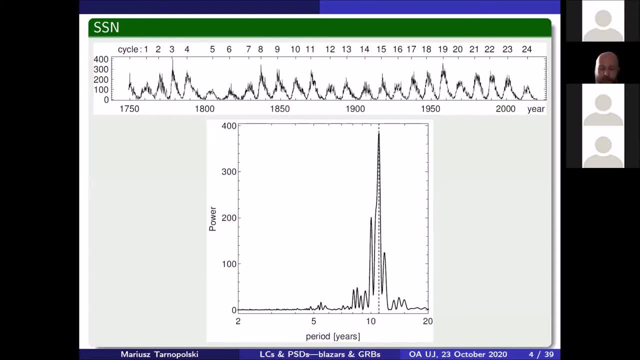 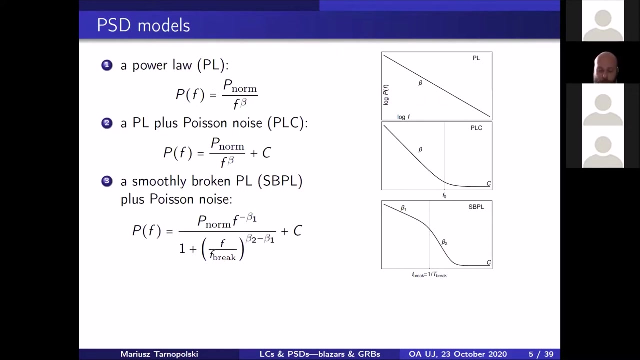 So this looks like this very convincing, and the LSP in general was actually designed with an application in identifying periodicities in stars or asteroids and so on, and works well here also, as presented Now. often one wants to examine the overall shape of the PSD and the most important example is the power law 1 over f to the 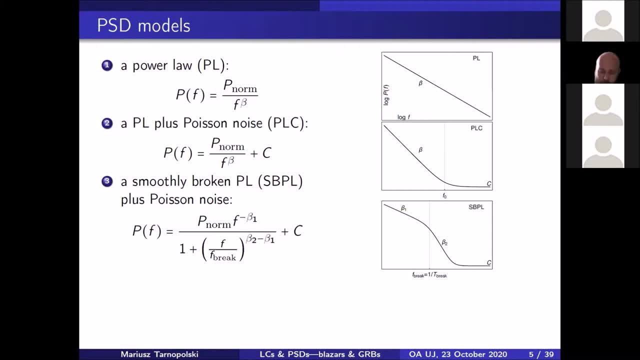 power of beta which in a logarithmic space is a straight line with slope. beta Frequently encountered is also a power law which flattens out above some critical frequency: f0. so there are two components in the PSD and above f0, the white noise dominates over the power law component and we 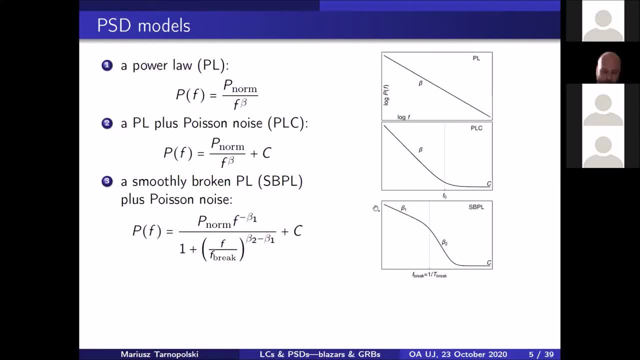 can see these in this: несколько reactions and two forces. DOM dominates over the power law and we can see these together in the next, already translated example. can also have a PSD consisting of two: power loss with a smooth transition from the low frequency index, beta 1. 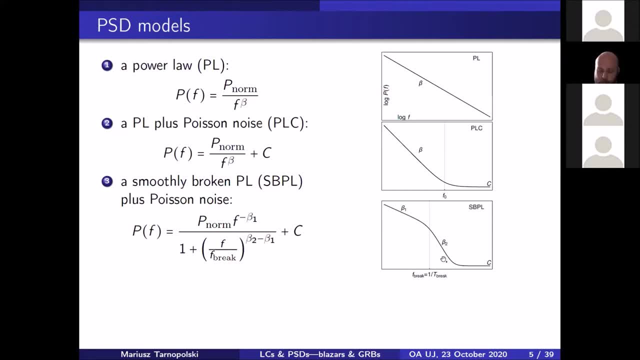 to the high frequency index beta 2 occurring and some break frequency And the constant C in these two cases is the so-called Poisson noise level, coming from the uncertainties in the individual measurements, That is, if one observes a value of 20 plus minus 1,. 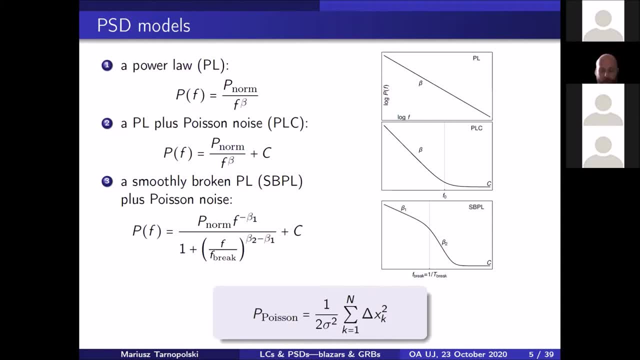 it can actually be slightly above or below 20.. Then let's say one observes 21 plus minus 1, which again can in reality be slightly off, though with a different magnitude or direction than the previous measurement. So these uncertainties introduce a bit of randomness. 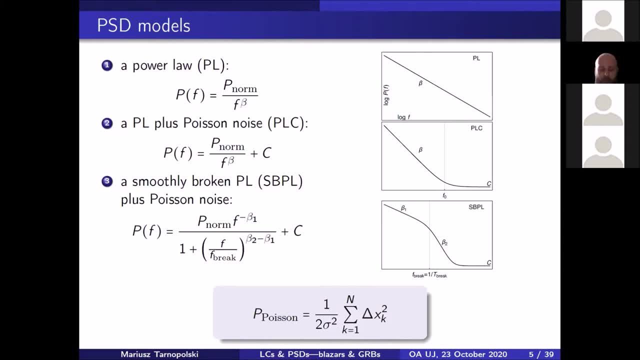 to the observations. This is an additional randomness, And the higher the noise level, so the bigger the errors, or the smaller the signal-to-noise ratio, to put it differently, the more the actual signal will be buried in the observational noise. So the Poisson noise is more often than not. 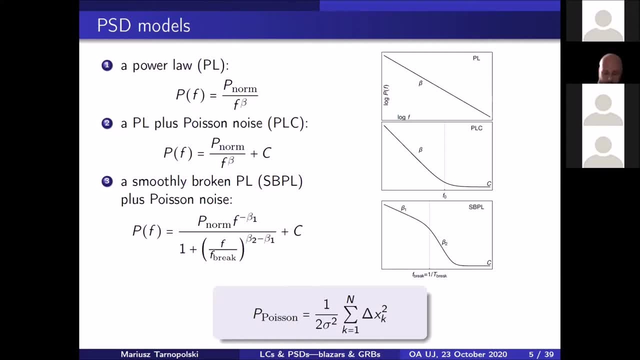 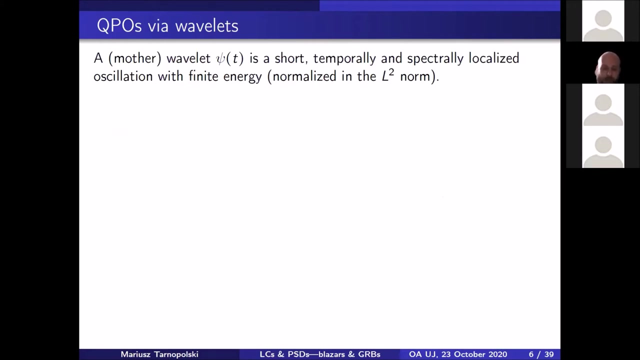 a limitation of the equipment or the background radiation of the sky that obscures the signal more for dimmer. So it's usually nothing really physical in the source itself. I mean this constant level C. So this was one thing. Let's go to wavelets, which in essence are wave packets. 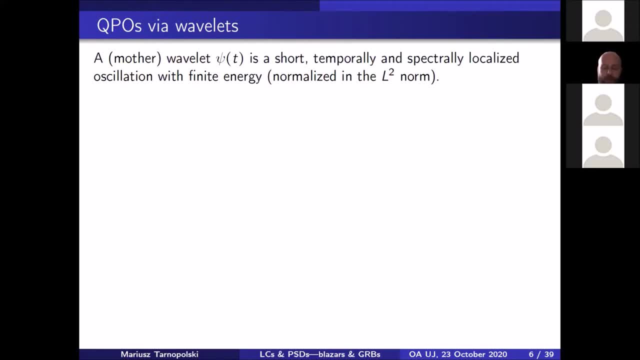 constrained in time, oscillations with a fixed primary frequency. So there is a bunch of different wavelets, which can be complex like this, More like this, More that wavelet where the real and imaginary parts are blue and red respectively, or this purely real hard wavelet. 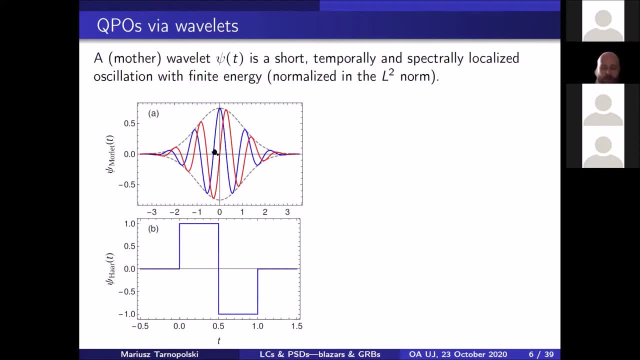 The more that wavelet is actually a cosine within a Gaussian envelope. And now, given a mother wavelet like this basic wavelet, one can form an orthonormal basis, called a dictionary and composed of, so to speak, So called child wavelets, by a translation and rescaling. 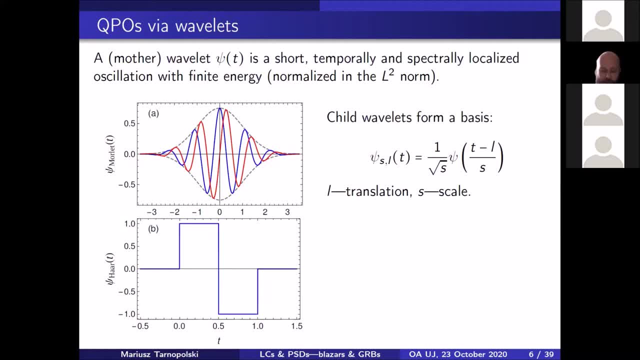 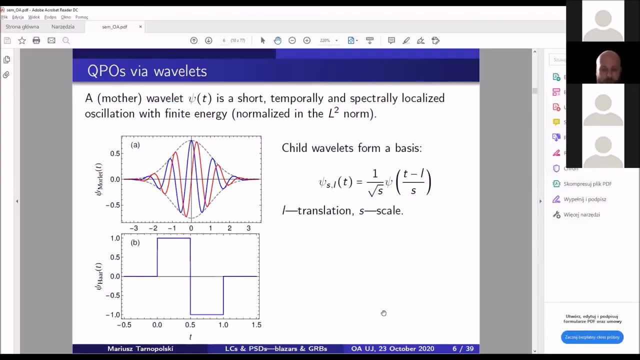 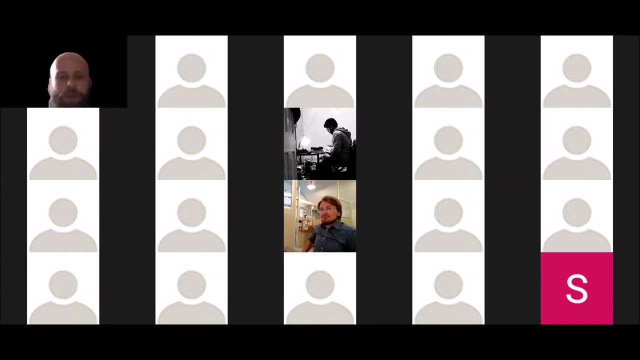 of the mother wavelet, And this is best illustrated by a demonstration that I will somehow need to switch to. So let me stop sharing for a moment, switch to another window and I'll go back to you. OK, This seems to work quite easy. 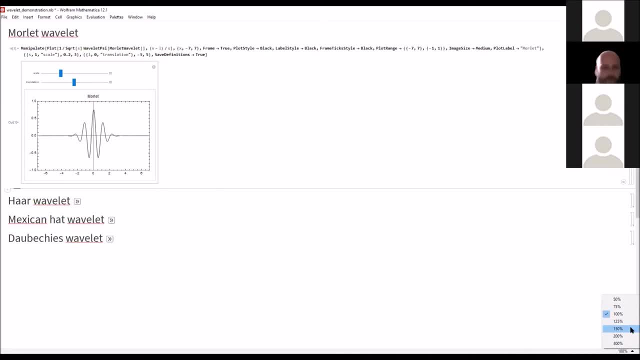 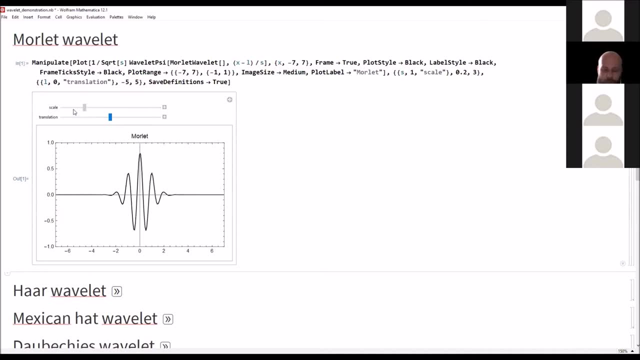 So do you see this? Yes, we do. OK, So everything worked Great. So the wavelet can be squeezed and expanded by changing the scale parameter and moved around left and right. translated as well, And the same applies to the other. 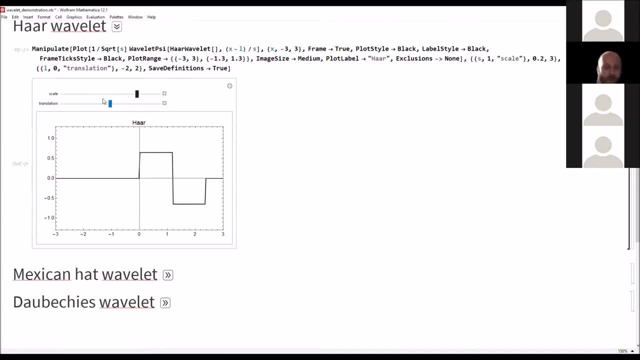 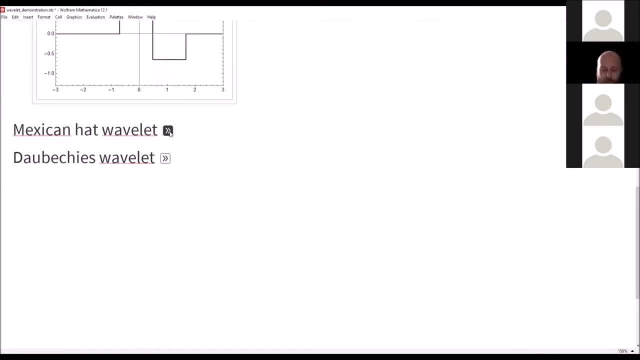 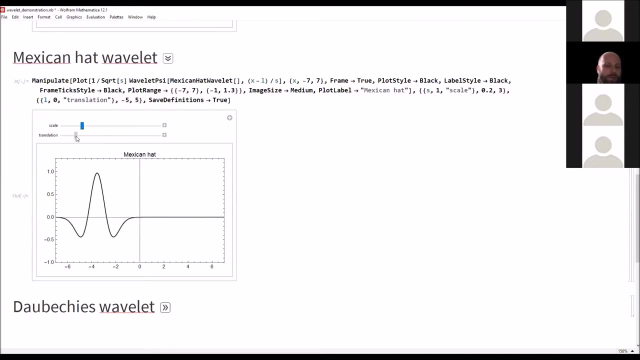 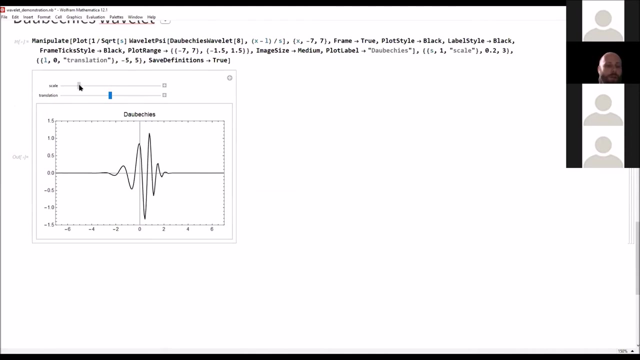 So we have the hard wavelet, which has a different rectangular shape, And there are also lots of other wavelets, like this so-called Mexican hat, or the whole family of the so-called Daubecci's wavelets, Yeah, and many more. 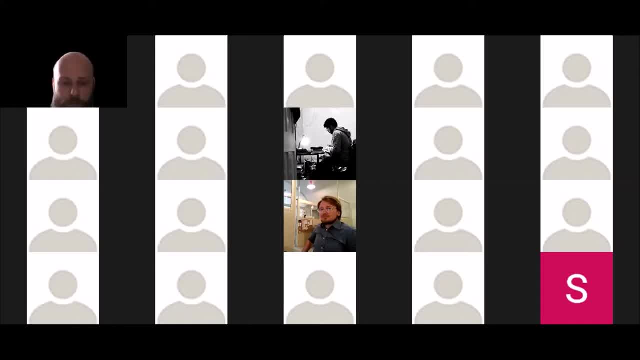 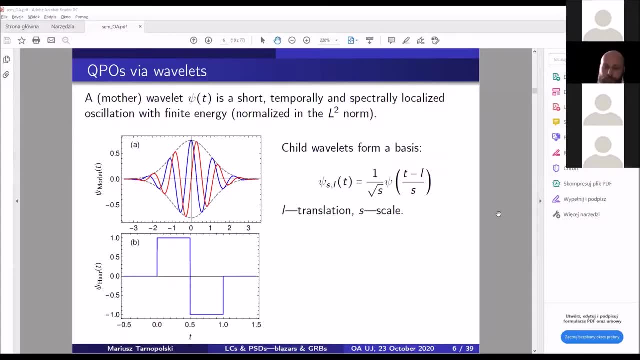 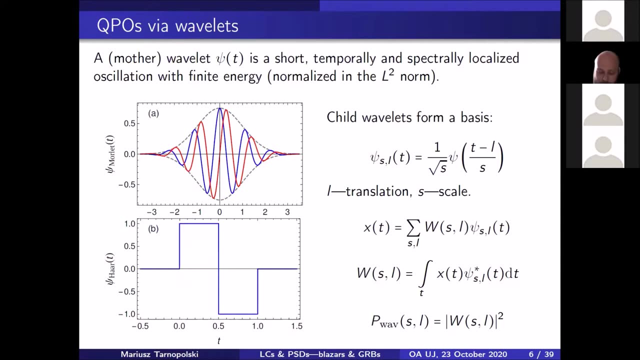 So again, first switch, OK. So, given a signal x, since child wavelets form a basis one can decode OK. OK, One can decompose the signal into wavelet components. This works similarly to the well-known Fourier case. 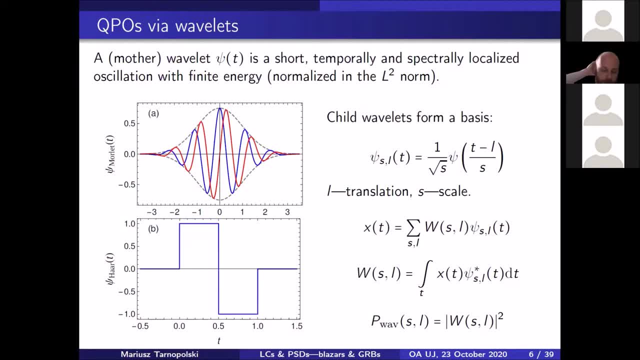 In the Fourier decomposition, one decomposes the signal into a combination of signs, each with different base frequency and with different coefficients indicating how much power is carried by a given frequency component. Here it is similar, just that instead of only the frequency corresponding to s? 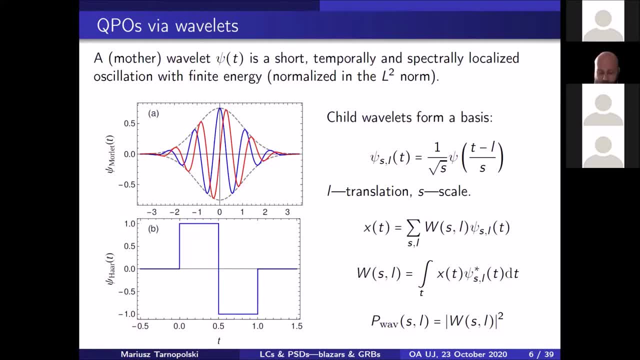 there is also the location l, And psi here takes the role of the e to the e times frequency, part of the Fourier transform which gives rise to the sign, which is actually infinite in the sense that it doesn't start at a particular point. 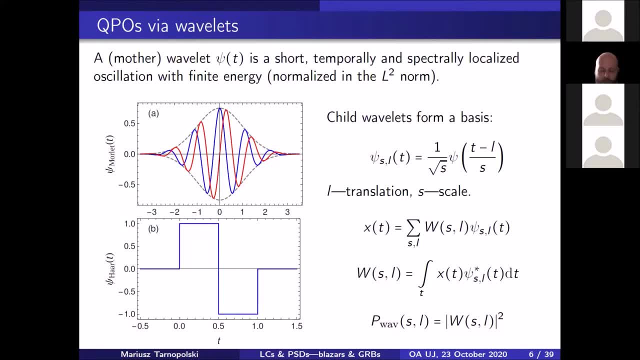 and then end being eternal while wavelets are localized in time. So if one put here: Just assign and drop the translation from the w coefficients, one would basically retrieve the Fourier transform. So the wavelet coefficients are obtained as an l-squared scalar product of the basis. 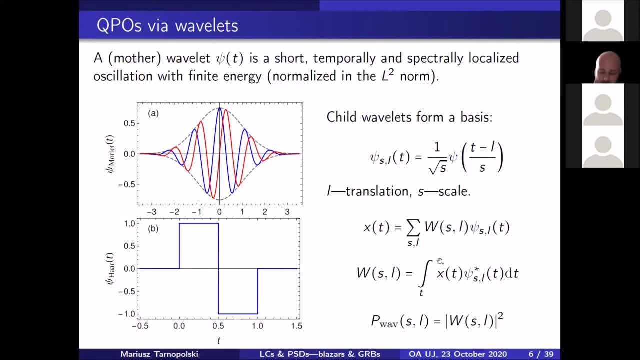 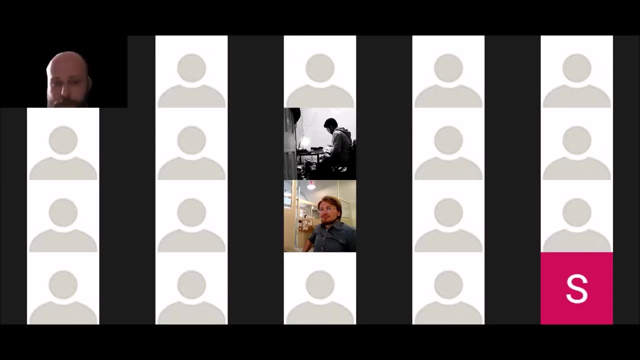 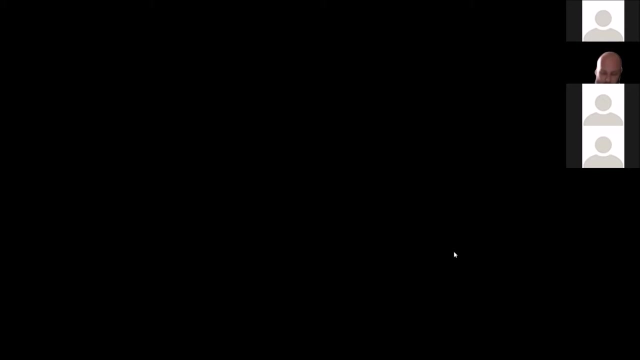 with the signal in the usual way. And then finally the power in the so-called wavelet scalogram. OK, It's obtained also as a squared modulus of the coefficients. And let me again switch to another demonstration. So let's say we have a signal that initially has: 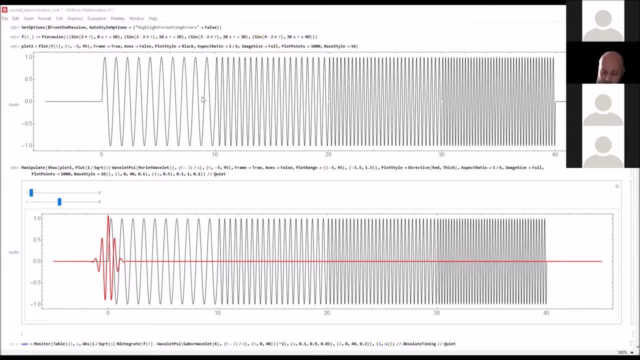 a frequency of 2 pi And after 10 units of time it doubles to 4 pi, Then to 6 pi And then to an 8 pi at the end. So if one did an LSP there would be four peaks corresponding to the localizations. 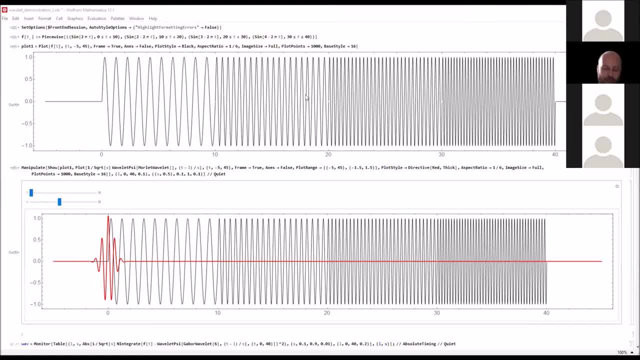 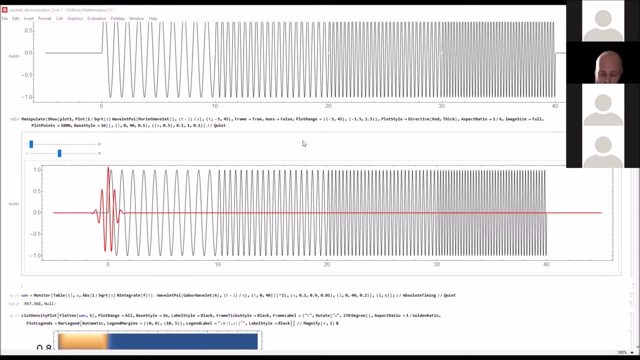 of the components And the constructed signal would be a linear combination of signs and not a chirping signal like this initial one. So what we do is take a wavelet with a given bar, with a given signal, And then we take a given scale and sweep it along the signal. 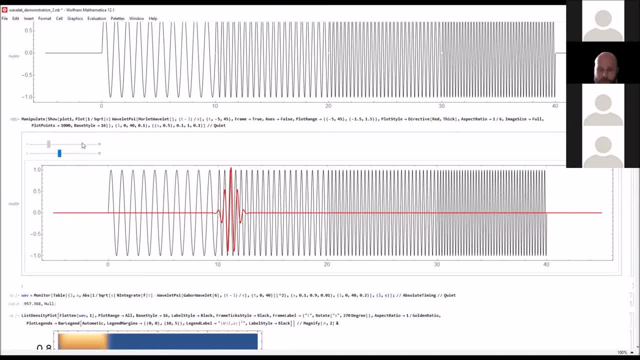 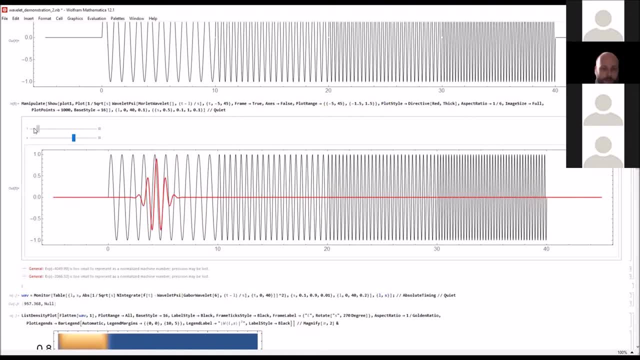 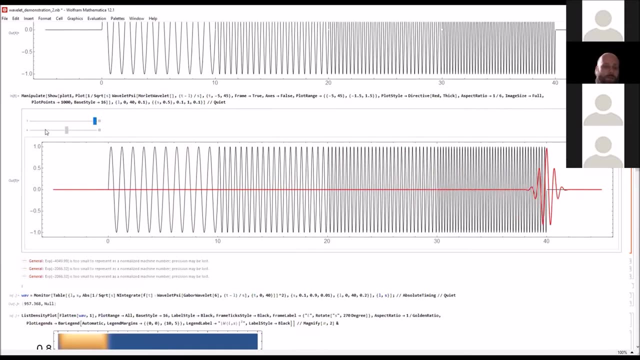 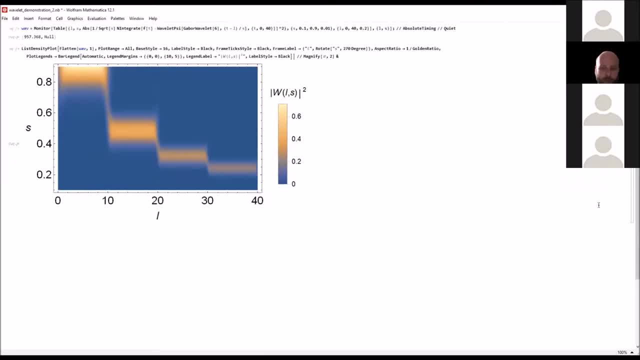 So in the end we can obtain a plot like this, showing that at times from 0 to 10, there was a signal with a frequency corresponding to some given s. s is actually proportional to the period, So it's the inverse of the frequency. 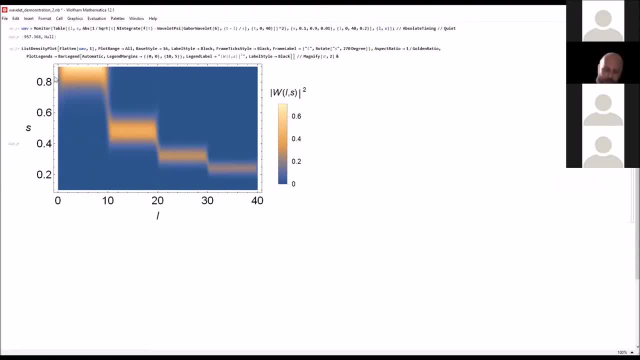 And the proper units can be figured out and normalized, But there is no power at later times at this scale, at times greater than 10.. But then again there is this segment when the power corresponding to some other s was high, and similarly for the next portions as well. 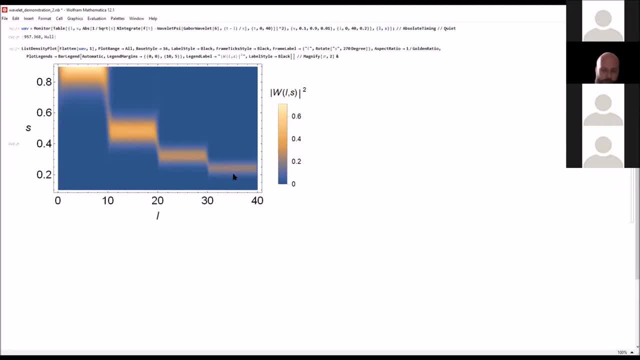 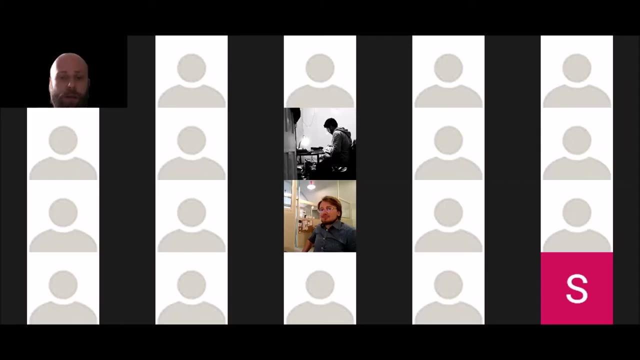 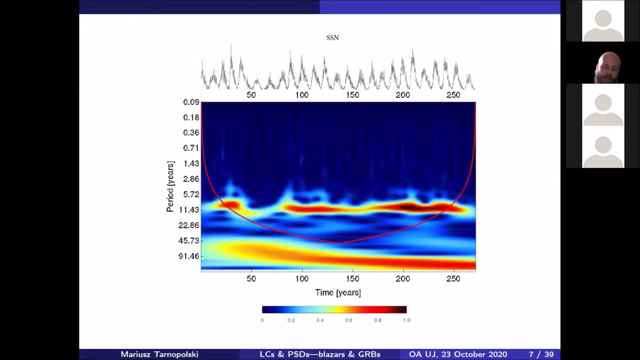 So one can see the leading period: overall decreases in time. So this is basically the methodology used also to examine fast radio bursts or the gravitational waves. And now I can go back to the presentation for the rest of the talk. So let's take as an example again the sunspot number. 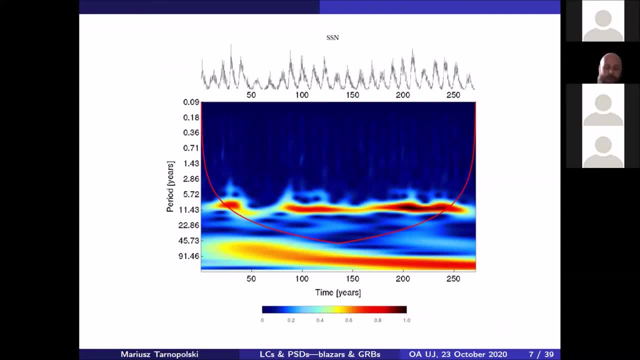 sequence, And there was a strong component identified at an 11-year period, And indeed, the scologram presents a more or less constant and persistent modulation throughout the time series. at about 11 years, Moreover, one can see a fall in power. 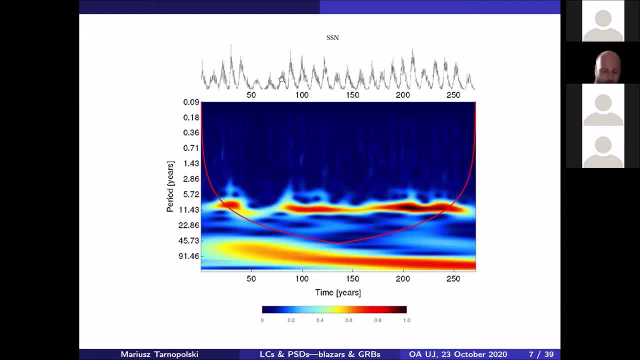 around here, which corresponds to the so-called Dalton gap. So a mindful examination of the scologram allows to deduce both the overall and minuscule behavior of the analyzed data. Moreover, we see here something at the period of 100 years. 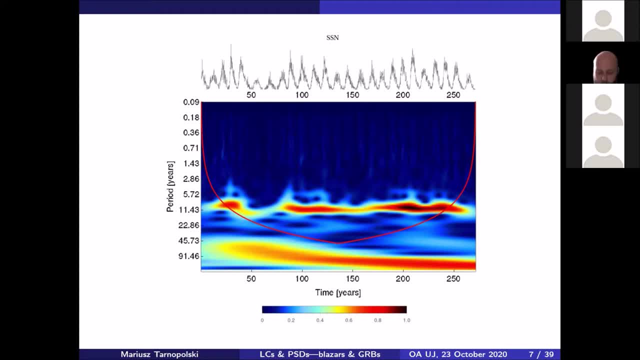 which, after a closer look at the sequence, looks like a sinusoidal envelope, like here in the upper part. So at the beginning of the sequence there's only part of the cycle Starting with low peaks And this is represented in the scologram. 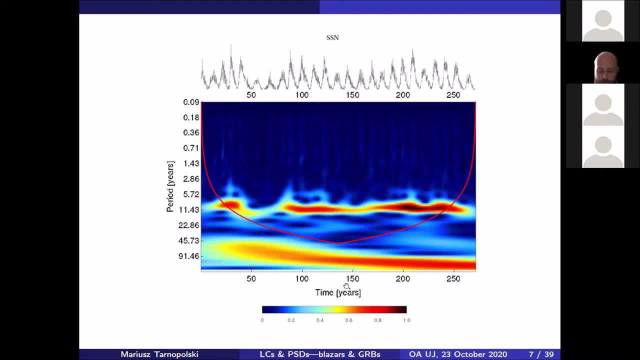 as a bend toward lower periods, And this red continuous line is the so-called cone of influence, which is actually the region below these lines, And it depicts the region where the finite length effects are significant, That is, the influence of the edges of the time series. 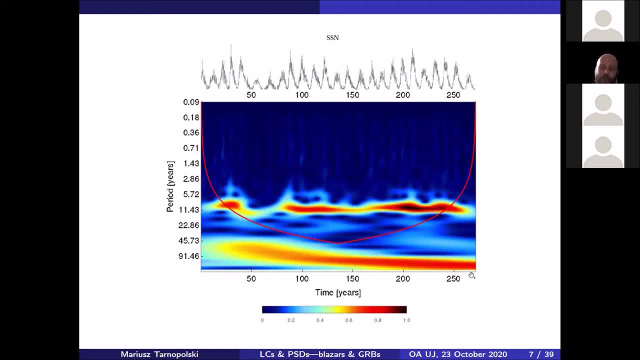 So to speak. So this 100-year cycle is there, but one has to be very, very cautious when interpreting it because of the cone of influence. So a longer time series in this case would lower the cone of influence. so one could then get a significant estimate of this 100-year cycle. 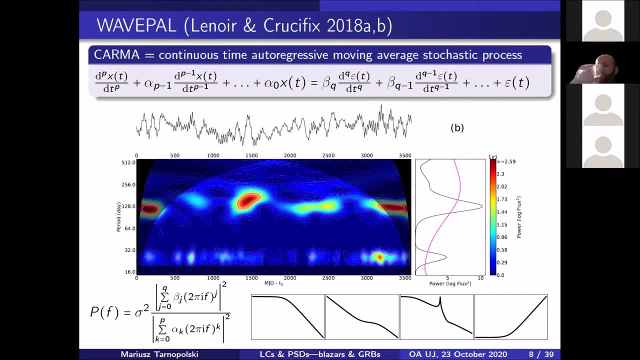 Yeah, Now, Sorry. OK. Now what is of importance is to assess which fixed features are actually statistically significant And when dealing with global periodograms like the LSP or Fourier, one simulates lots of stochastic models believed to underline the overall observed PSD. 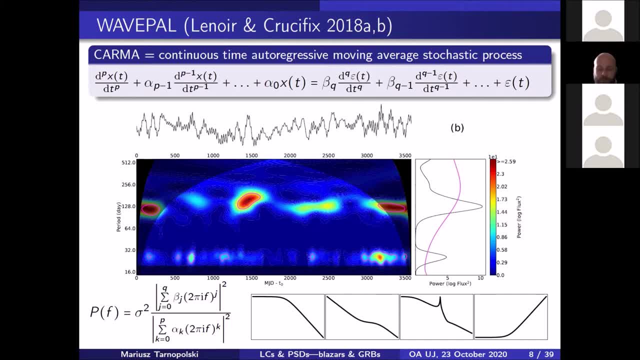 and then checks which spectral features in the observed signal exceed some given significance. So H- And a very good reason is to estimate the quantum intelligence of the 0- is equal to the challenge to actually get the result from the reference level, hopefully at least 3 sigma, say. 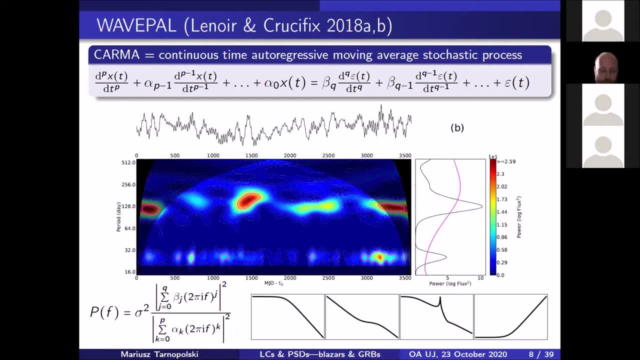 One could in principle do the same for the Scalogram, and the method we employed, implemented in the package wave PAL, which is suitable also for highly irregular time series, applies a so-called Karmas Stochastic model as the background model for the variation. 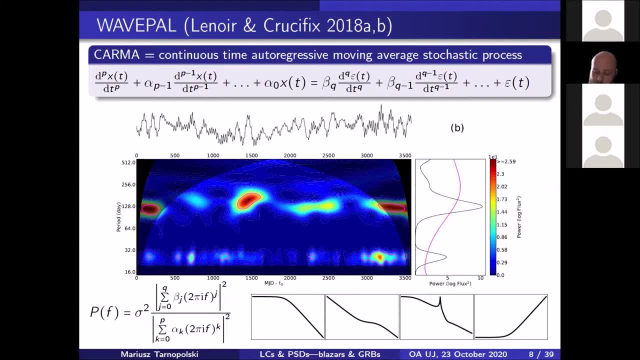 Karmas stands for continuous time autoregressive moving average, So it's basically a continuous time AMA And it's basically a continuous time ARMA. It's not crucial here to go into details, but CARMA's PSD is quite flexible. 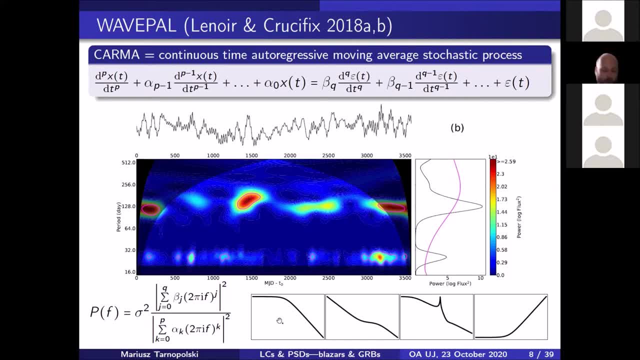 It can be either a Lorentzian or a white noise transiting to a power law. It can contain spectral breaks, peaks or some other weird features as well, And the magenta contours on this collogram here denote the 3-sigma significance level. 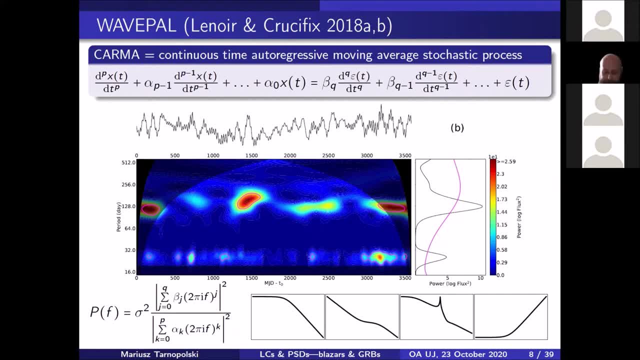 against the best fit CARMA model. The signal itself here is just a mock one with implicit long and short term periods roughly revealed here at these bounds below 30 days and about 100, something like that I will demonstrate later. The signal is important to highlight the interesting features, to deal with the non-stationarities. 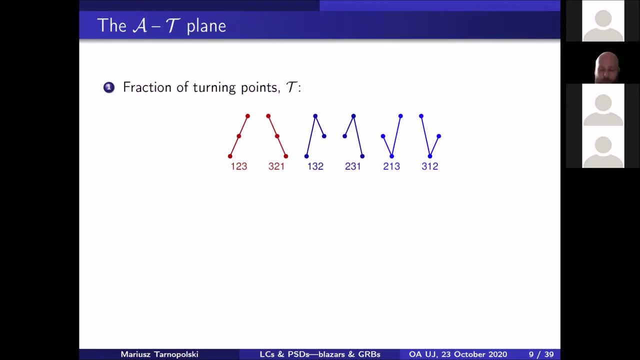 And the last method that I'd want to talk about is the AT-plane spanned by the fraction of turning points T and the upper value A. A turning point is a point where there is a swing from an increase to a decrease. Okay, 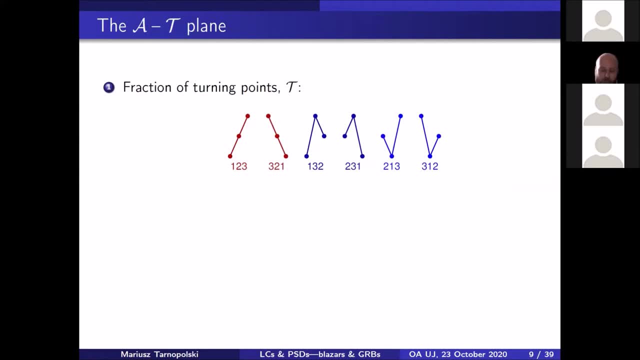 It's a point where there is a decrease, or vice versa. So these two blue peaks and these two valleys are turning points and these two reddish segments are not. So, having three consecutive points, one can arrange them in these six ways For the white noise sequence. all of these are equally probable because each point is 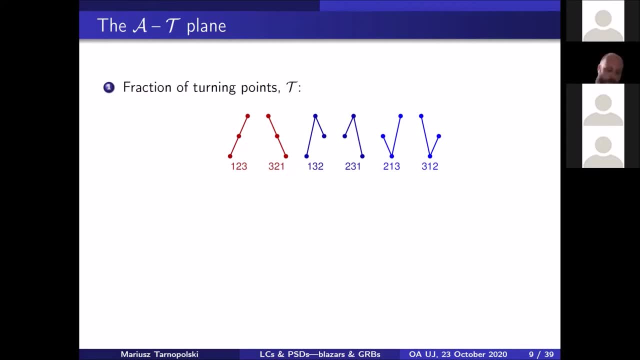 independent on any other. So the expected value of T is two thirds. Now, in general the probability of each point is two thirds. The probability of each pattern can be very non-trivial, like in the ARMA processes or power laws, Brownian motion, et cetera. 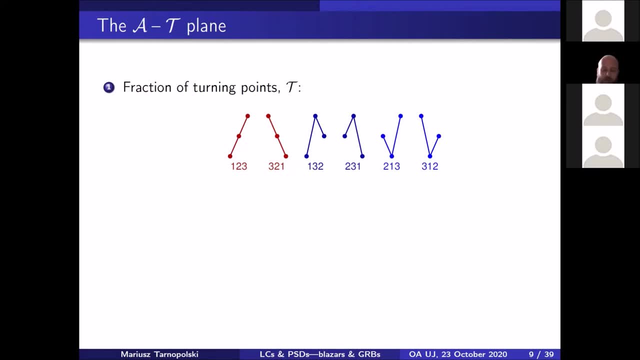 So T can be quite different from two thirds, ranging from zero when the whole sequence is monotonic, to unity, when the series is strictly alternating but not need to be periodic or ordered in any way. It can be also chaotic, So one can say that a series with T greater than zero is a series with T greater than. 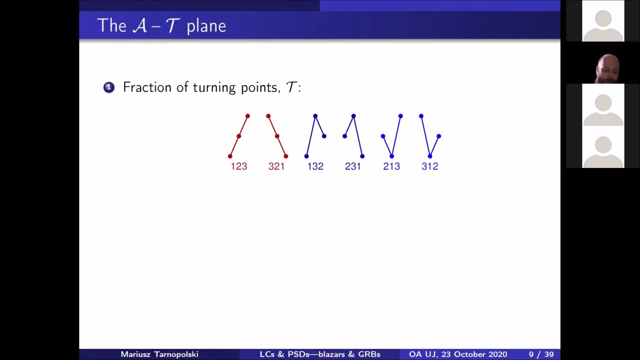 two thirds is more noisy and with T, less than two thirds is less noisy than white noise by comparison. And the Abbe value in turn is the ratio of the mean squares' successive difference to the variance. The successive differences actually form a difference series. 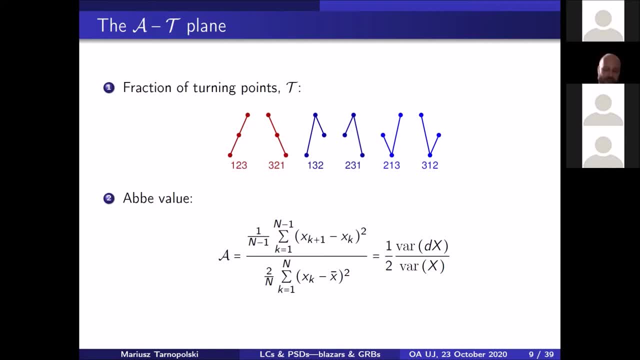 That is a series of differences, And hence it can be written as a ratio of the variance. Okay, So the variance of such differentiated series to the variance of the original series. So this is some form of a gradient, And A is normalized so that it's equal to one for white noise and can range from zero. 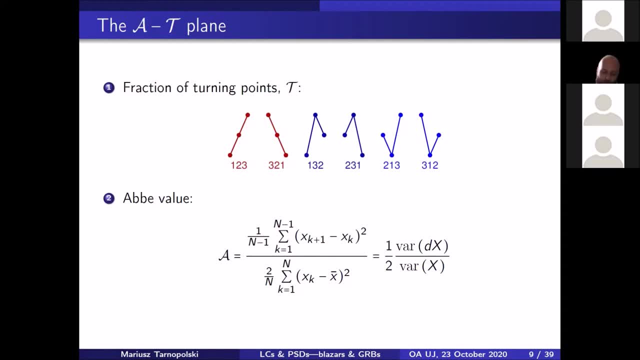 to two, And again A greater than one can be called more noisy than white noise, like the similar to the T case, And A smaller than one is less noisy than white noise, So it's less noisy than white noise. And finally, both A and T attain small values for very smooth curves and high values for 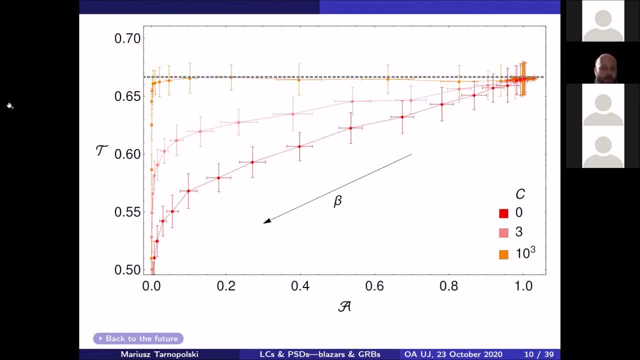 very rough or jagged ones. So to illustrate this, let's take simple power gloss. The red line here corresponds to pure power gloss, with increasing values of the index beta leftwards, And when it increases the path in the AT plane it increases the path in the T plane. So it's less noisy than white noise. So it's less noisy than white noise. And again, A greater than one can be called more noisy than white noise. So it's less noisy than white noise. And again, A greater than one can be called more noisy than white noise. 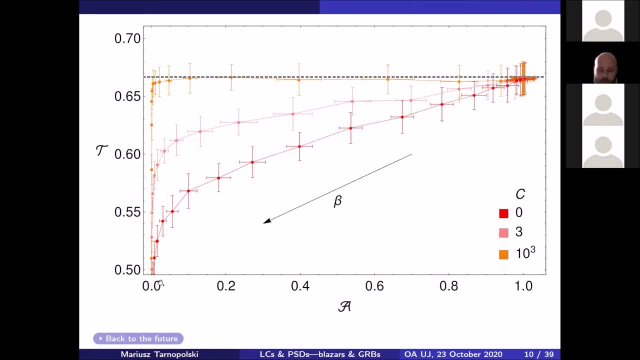 So it's less noisy than white noise. So at the case of pure power gloss, the vector light curvature of include yellow is less noisy than the V. perpendicular to C plane is curved and goes to the regions of higher smoothness. When some white noise is added, the paths and the corresponding points with the same. 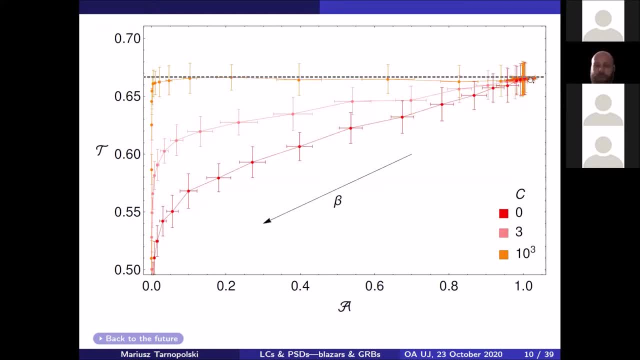 beta are rised and dragged closer to this point corresponding to white noise. This makes sense since when white noise is injected in the data, it will alter the probability of obtaining a turning point and will affect the gradient, the ruggedness of the series. 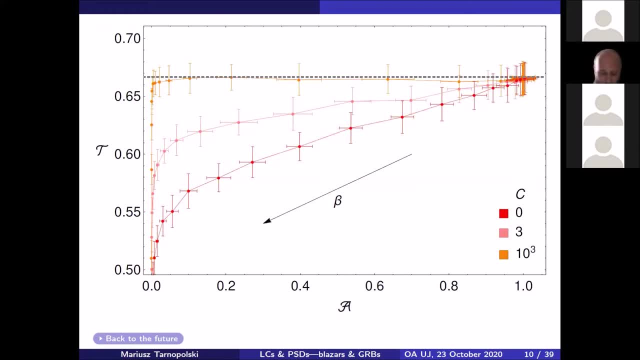 But even for a high level of white noise, when t is close to two-thirds, the values of a can be very different, hence allowing for, for example, classification, And indeed this method has been already successfully used in classifying global markets, diagnosing heart diseases or even 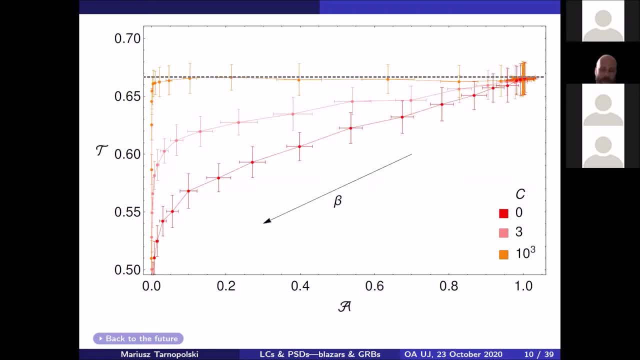 discerning patients with epilepsy. It turns out to be so sensitive that, in one study, it was able, for the very first time, to discern if the patient had open or closed eyes, based only on the EEG reading. And, moreover, it is prospective in distinguishing chaos from noise and regular behavior as well. 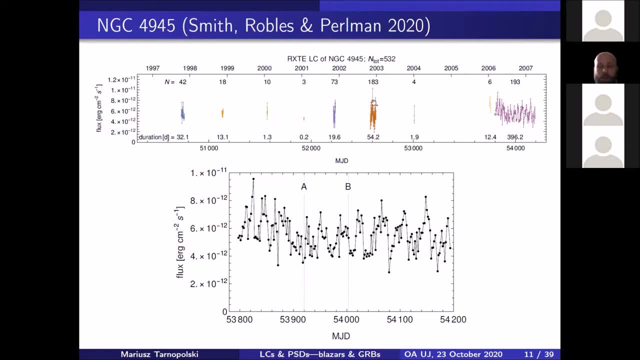 Okay, so that would be the introduction, And let us now consider as an example a very recent finding from just a few weeks ago of a group- Smith Robles and Perlman- who analyzed the RX-TE X-ray light curve of this: 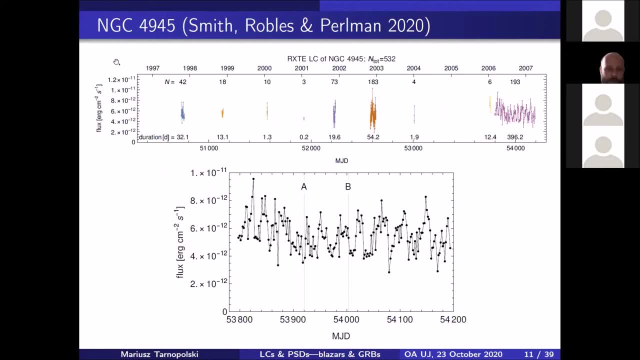 Seifert 2 galaxy, NGC 4945.. And this in the upper plot. this is the whole available light curve and it has different values. It has different segments, but let's focus on this last one with the longest span of over a year. 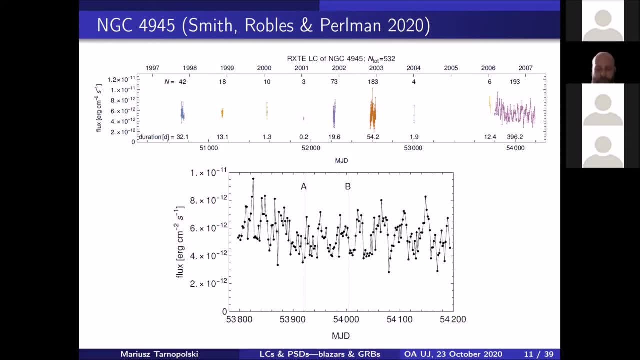 and almost 200 points. It is irregularly sampled with no big gaps within And in the lower part. there is the magnification of this part and one can see there seems to be some recurring variation in it. So one way is to just look at it. 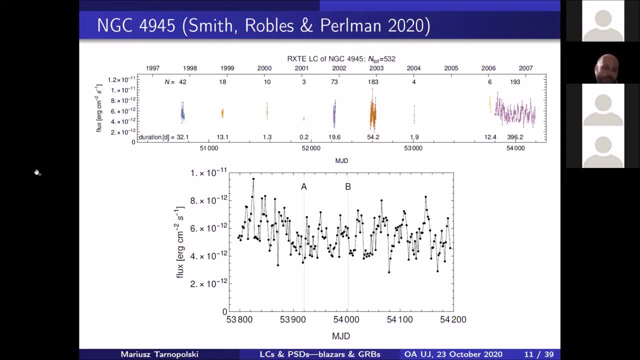 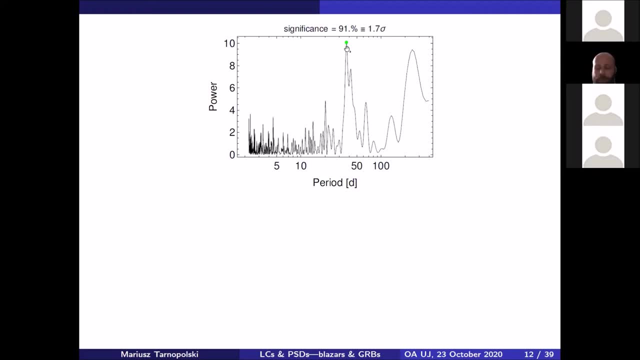 Just to feed it to the LSP and see what happens. And if we do it well, we've got a peak okay at the period of about 37 days, but its significance is only 1.7 sigma, So it's way too low to consider it a QPO or a discovery of anything. 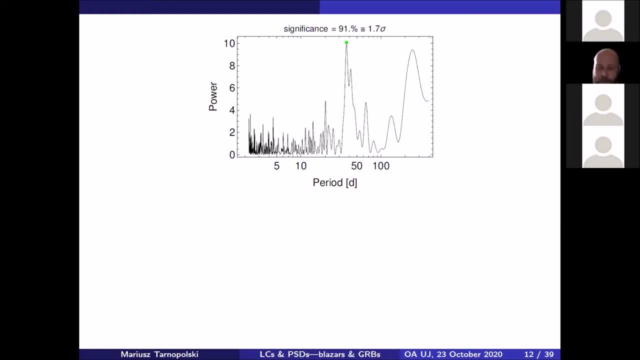 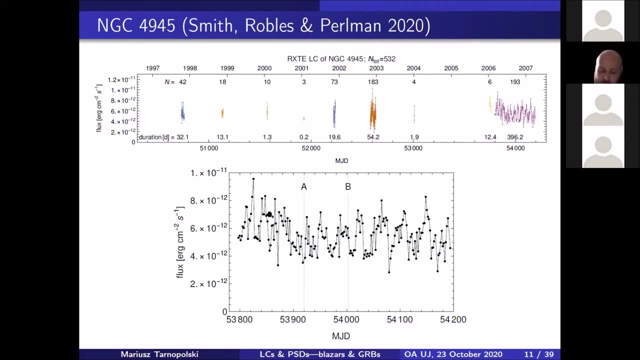 But let's take a look at the light curve again. At the beginning we have a quadratic kind of segment which is a downtrend. So maybe let's just take only the part after point A here, so everything right works. 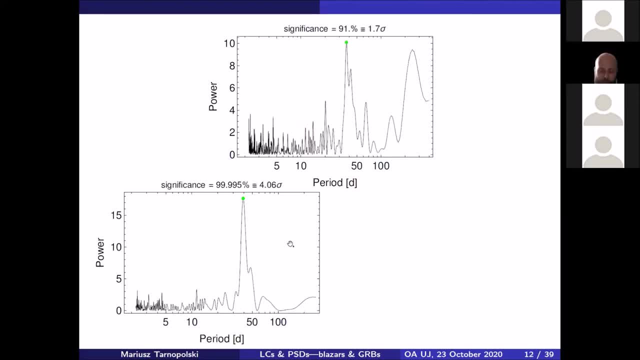 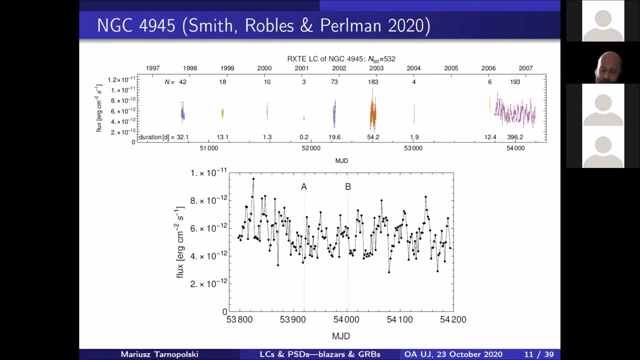 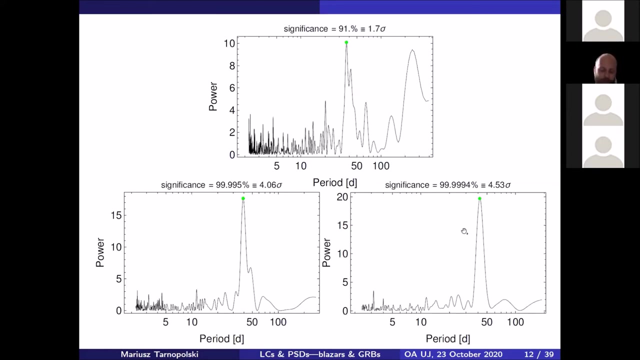 And indeed in this case we now see a peak with a considerable significance about 4 sigma. But actually the authors themselves considered the last segment, starting from point B here, lasting about 190 days, And the LSP of this part reveals a peak with about a 4.5 sigma significance. 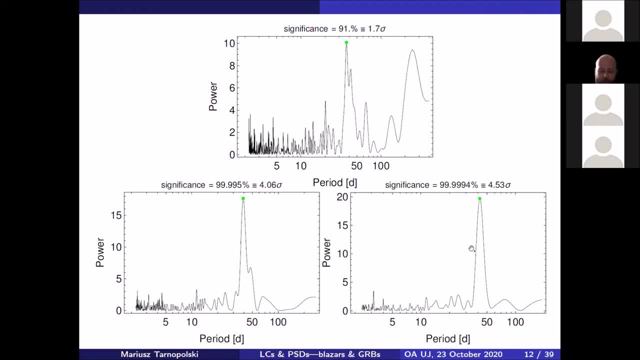 So all good, there is a peak. But this was like. one needs to first locate the QPO region to even detect it using the LSP. So that seems to be a very efficient and robust way. But now what obviously comes to mind are the wavelets. 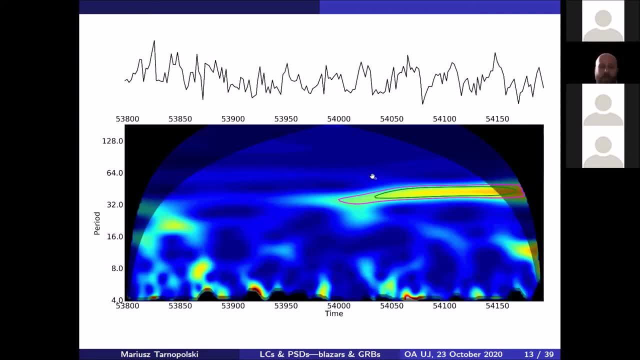 And indeed there is this nice constant and quite persistent modulation visible here at the 3 sigma significance And starting also roughly at about point B. like the authors isolated. But this gives an immediate overview of the whole thing. This gives an immediate overview of the whole spectral structure of the examined light curve and the significance level too. 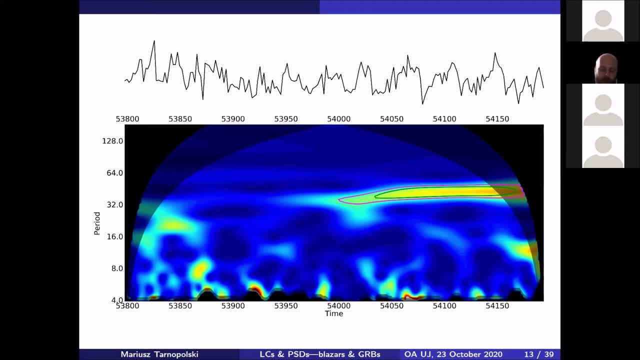 Actually I haven't seen a scologram with contours depicting statistical significance in the astronomical literature, Just the analysis of the LSP and then showing that there is a feature in the scologram computed with another implementation that we are using here. 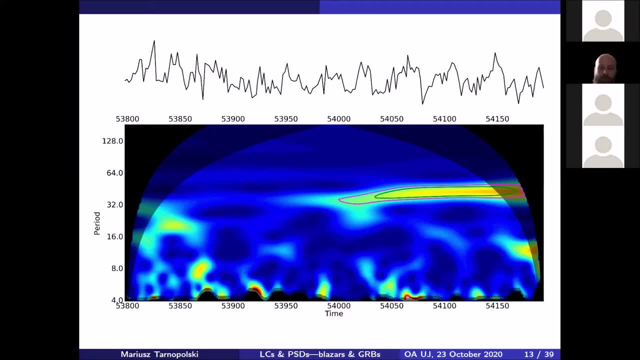 But then again, the significance of the LSP and on the scologram are different, As the latter, on the scologram, is smeared over a two-dimensional plane, while the global periodogram is a projection of all the power at a given frequency on the vertical axis. 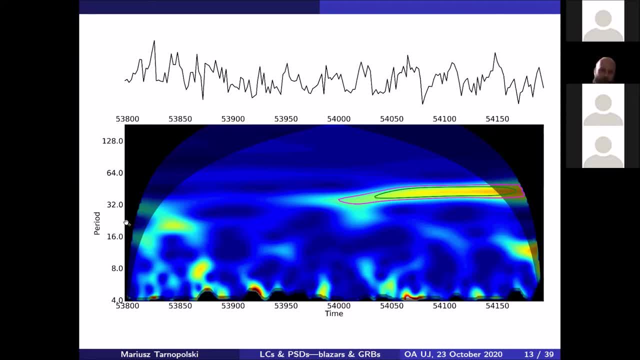 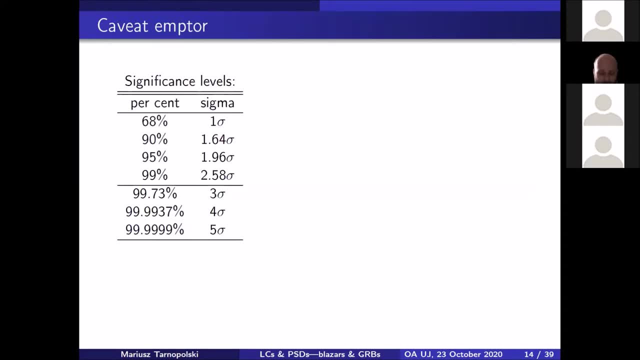 So, in short, wavelets are a powerful tool in analyzing the PSD and searching for some features. Now a note about the significance. I think it's well known that one sigma corresponds to 68% and that two sigma is roughly about 95%. 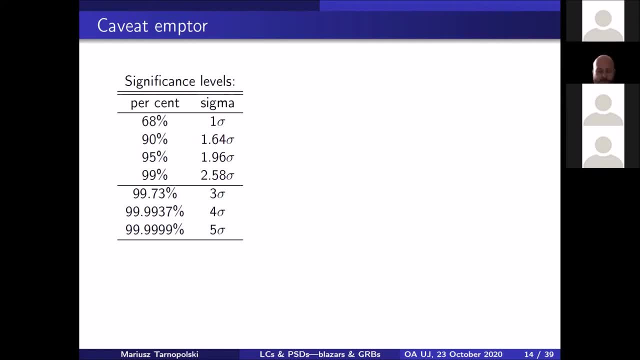 But in everyday life, when we say that something is 99% certain, such a high percentage virtually symbolizes certainty, Like if one would know that tomorrow there will be 99% certainty or 99% chance to be injured in a train accident. 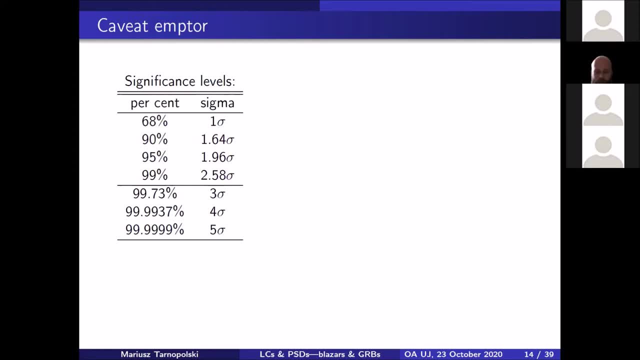 well, he wouldn't go near the railway at all, While on the other hand, if there was a 99% chance of winning millions in a lottery, the ticket sales points would be stormed with buyers. But in fact, 99% is just merely just over two and a half sigma. 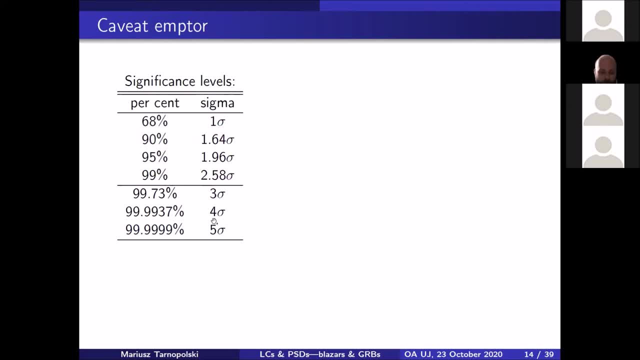 And basically we need more like three, four or five sigma to talk about the reality of a phenomenon. And let me illustrate this with a story. In 1976,, an LHC team led by Leon Lederman, a later Nobel Prize laureate. 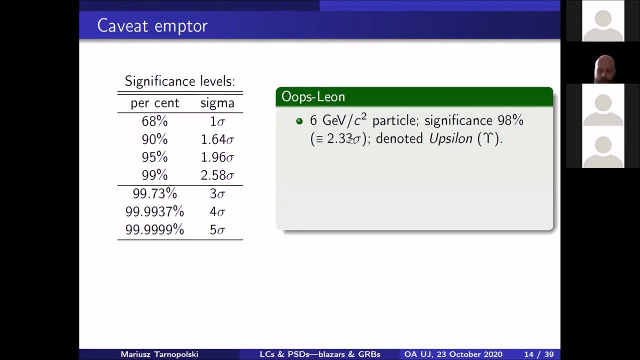 announced in physical review letters the discovery of a 6-GEV particle with a significance over 98%. The paper actually used a phrase- one in a 50 chance. So they gave the particle a name- epsilon, But only a few months later. 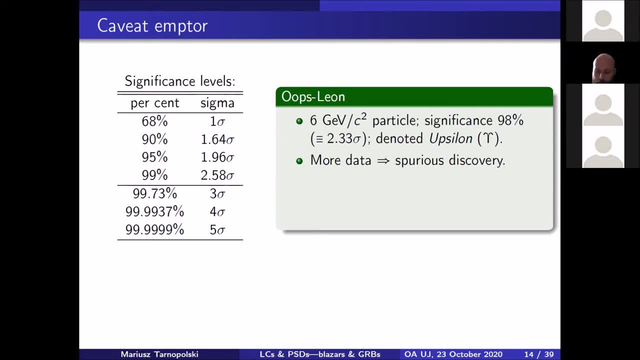 when more data was accumulated, it turned out, this presumed particle vanished in the noise. So the mere 2.33 sigma significance changed the premature epsilon to the now known oops. Leon Pan to Leon Lederman, But later. 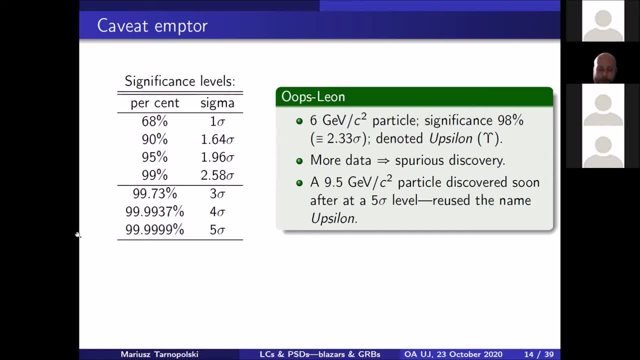 only the next year, in 1977, the team published the discovery, all this time on a five sigma level, of a nine and a half GEV particle, and they owned their previous mistake by using the name epsilon. So the epsilon is a real resonant particle. 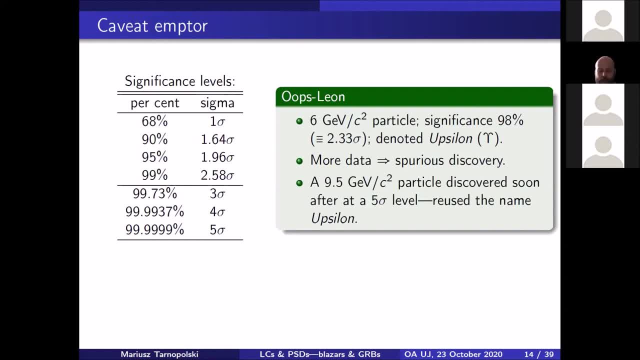 while an oops Leon is a discovery that doesn't exist. So since then, in particle physics, the five sigma level is an ultimate must, But in astronomy we generally use the same principle when it comes to discovering sources like gamma ray emitters or radio sources. 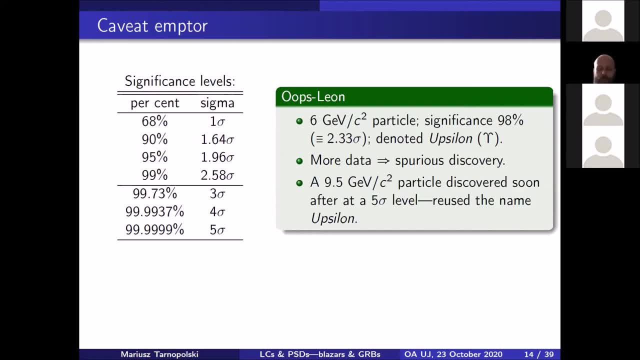 I mean to assert them if the source is even on the sky or not. But curiously enough, when it comes to detecting transient phenomena, the required level is greatly lowered, sometimes with detections being claimed at a less than three sigma level. 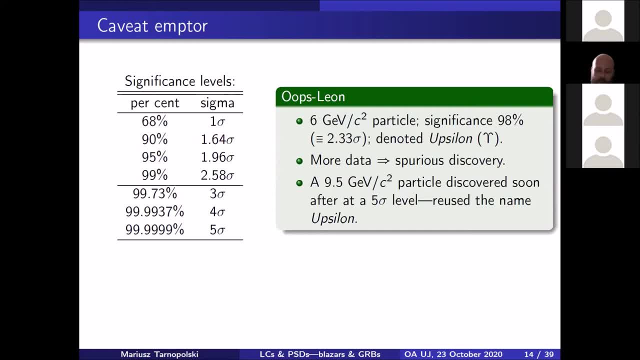 And actually invoking a five sigma level would conform to the standards of the discovery, although there would be very, very few QPOs discovered on such a level, maybe just one or two, even while the three sigma level should constitute a candidate. 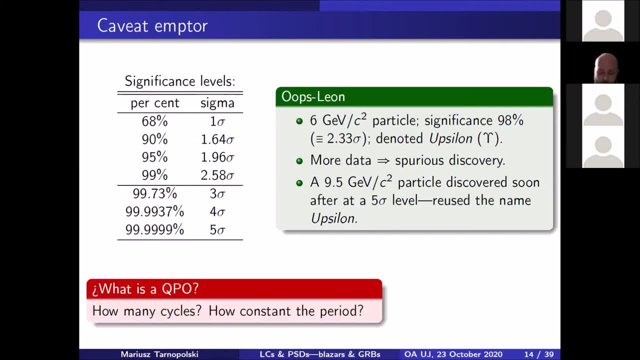 So, either way, there is also this other issue: What actually is a QPO? I mean, it's an oscillation, It's periodic, but not precisely, because it's quasi meaning, similar to, but not exactly. So let's say, there's just one cycle. 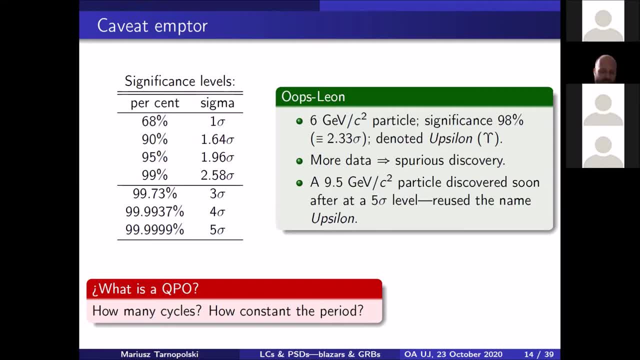 one bump in the light curve. So basically, this isn't a QPO. It could be anything- a flag, a glitch, anything really- But then if there's only one, where's the periodicity in it, since it doesn't repeat even once? 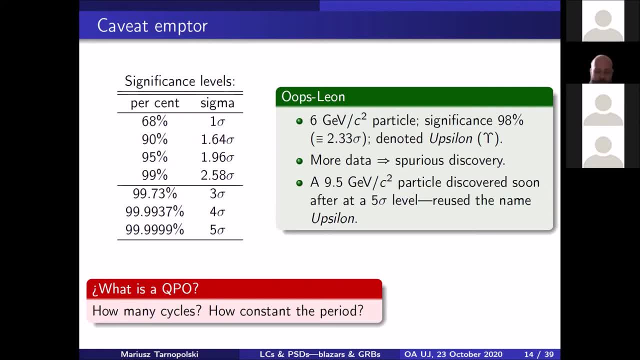 So that seems clear that more than one cycle is required. What if there were two? This seems recurring, but at what odds? Then they say, three is a charm. but since we always want more and more data, maybe we should require four or five cycles or more. 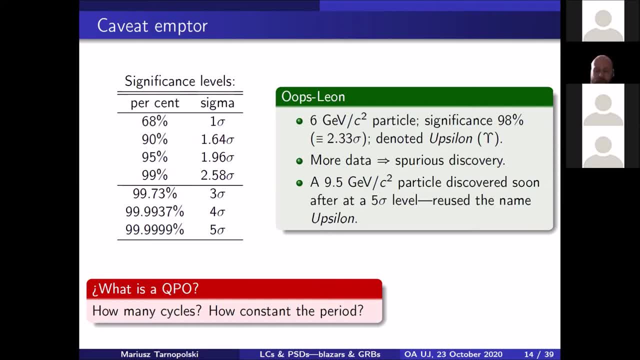 But then again, on the other hand, we are facing a barrier because QPOs are usually transient, in the sense that they start, last for some time and then fade away. So some phenomena, like gamma ray bursts, may inherently prevent us. 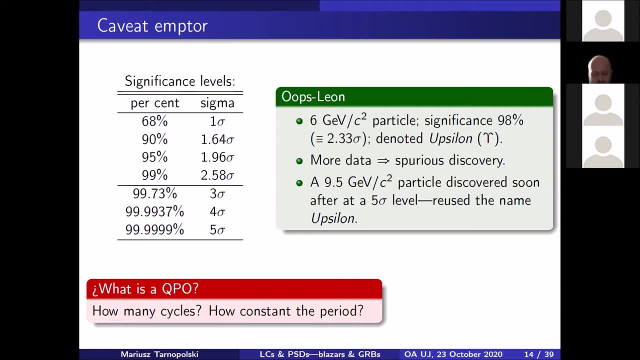 from obtaining a high significance. On the other hand, also, how constant do we require the cycle to be? Let's take, for example, the gravitational wave from a merger. This is an oscillation with a decreasing period, and then it abruptly ends at the merger. 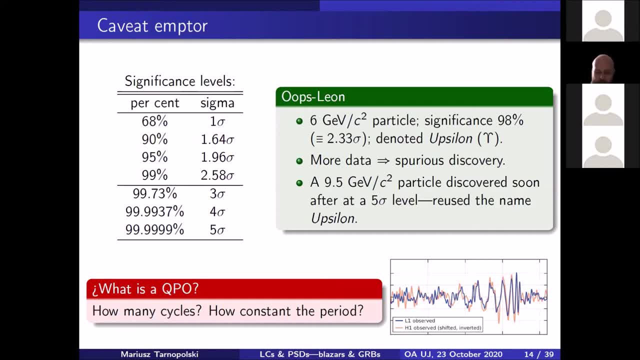 It's usually called the chirp or a chirping signal. So we can think this way: You observe a neutron star orbiting a black hole and you look exactly in the plane of the orbit. Every revolution you see, basically exactly the same image. 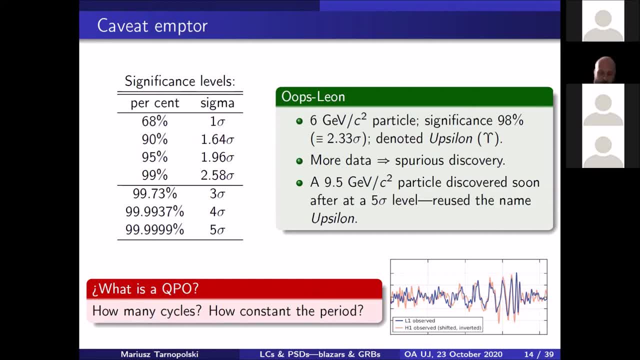 a neutron star in front of the black hole. Half an orbit later, the neutron star will hide behind the black hole and then you will see the same image again. So basically, every one revolution, the configuration is exactly repeated. So this is definitely. 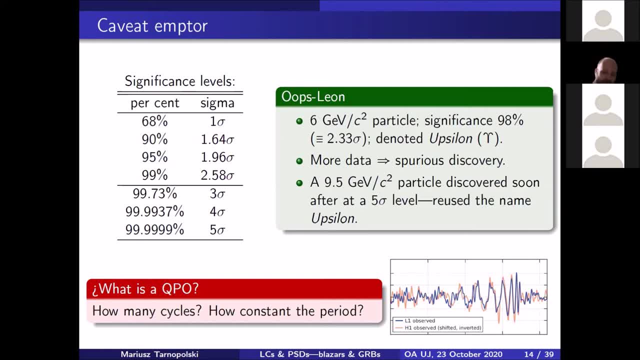 some kind of a recurring phenomena and maybe some kind of a QPO, And I don't have a particular answer or a recommendation here. This is something that basically should be debated in the community. I mean the proper definition of a QPO. 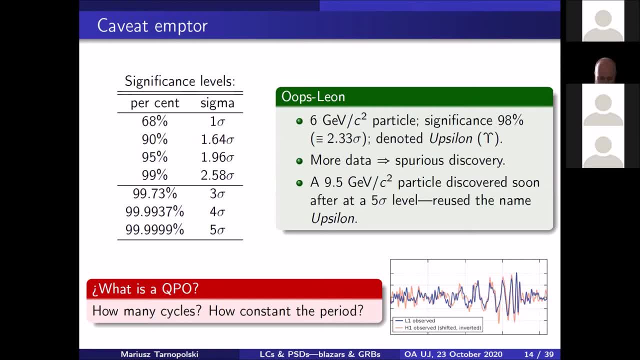 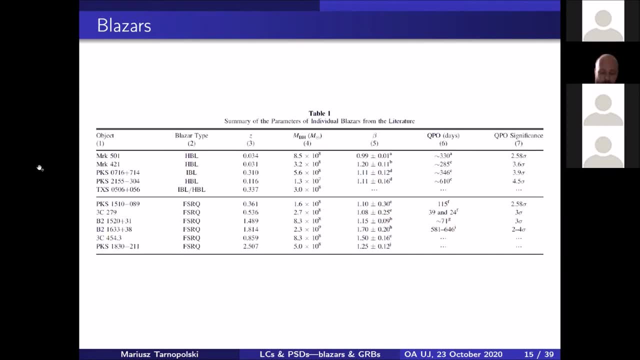 like what we are actually really looking for. So let us now proceed, finally, to some actual results. Recently, in a paper of ours, we analyzed in great detail the Fermilab gamma ray light curves, spanning 10 years, of 11 of the brightest. 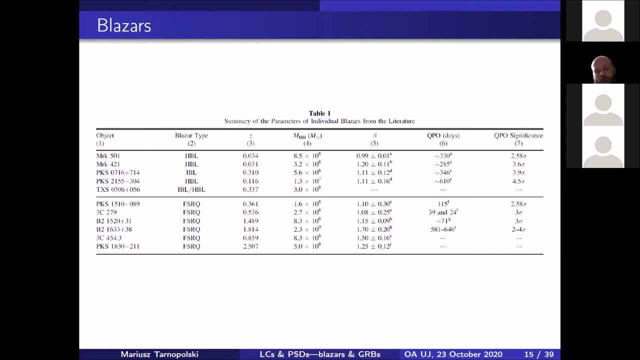 or otherwise famous blazers like Mach-Agen 501 or 3C454.3,, using a variety of methods and performed also exhaustive benchmark testing of their reliability. I obviously don't have time here to describe everything in detail, so this will be just about. 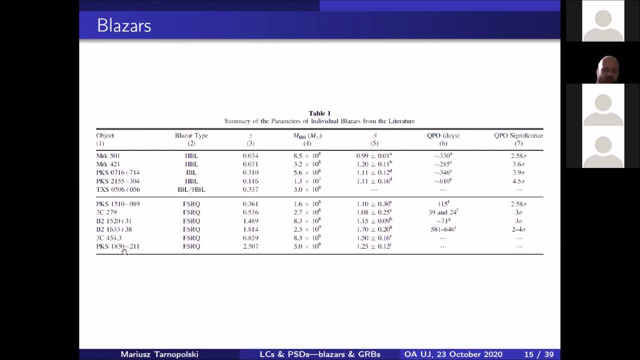 a few of the selected results. Anyway, there were five BL-LAC type objects in our sample, including the famous neutrino emitter TXS0506, and six FSRQs, including PKS1830, which is a gravitational lens in the gamma rays. 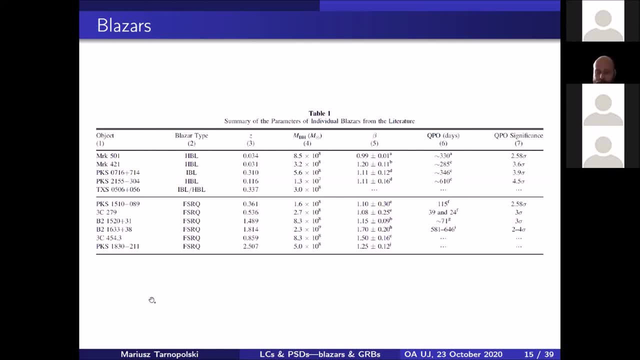 In eight of these 11 sources. some QPOs were already reported in the literature, though with quite various significance, from below 3S, sometimes reaching something like 4 or 5S, And the power law states that these shapes have beta indices falling mostly. 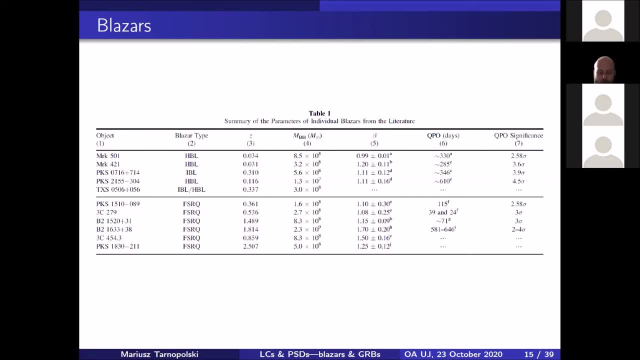 in the range between 1 and 2.. Sorry for interrupting, but these are the QPOs reported strictly for the Fermilab light curves or in general. No, no, no, these are strictly Fermilab, No optical, no X-rays. no, nothing else. 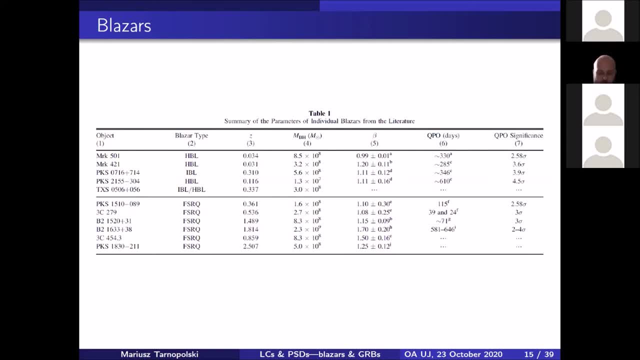 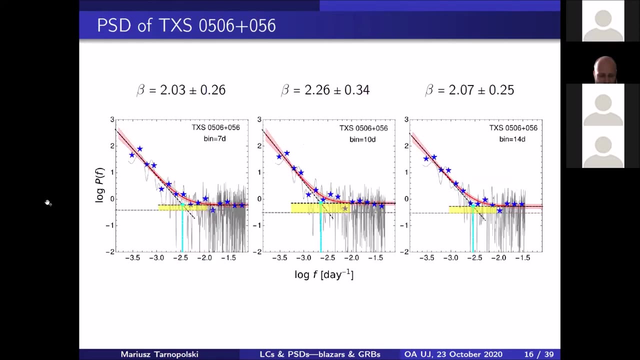 Okay, thanks, Yeah. And regarding the beta indices, this neutrino emitter, the TXS source, hadn't been examined in this regard. So, basically, this is how the PSD looks like for that source, with beta roughly being of the red noise type. 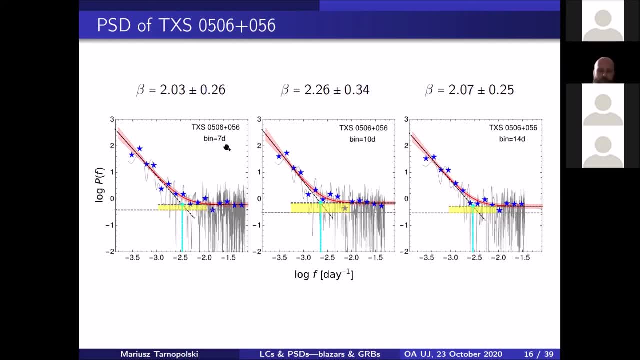 And to clarify, we analyzed three versions of the light curves for each object with a 7,, 10, and 14-day binning. That is the time step between the observations in the binned light curves, just to ensure the consistency of the obtained results. 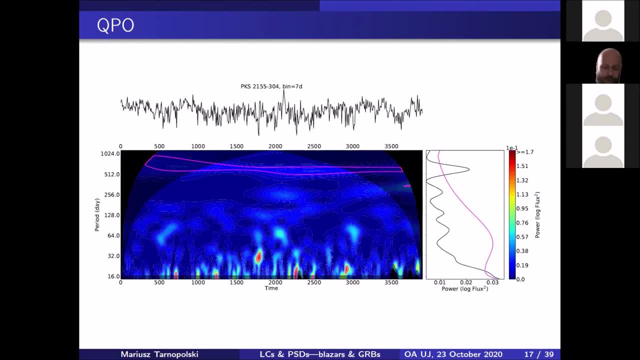 And regarding the QPOs per se, we confirmed the quite famous 600-day QPO in PKS 2155 with a percent 3-sigma modulation throughout the whole light curve. Compared with several previous works, there has been a gradual decrease. 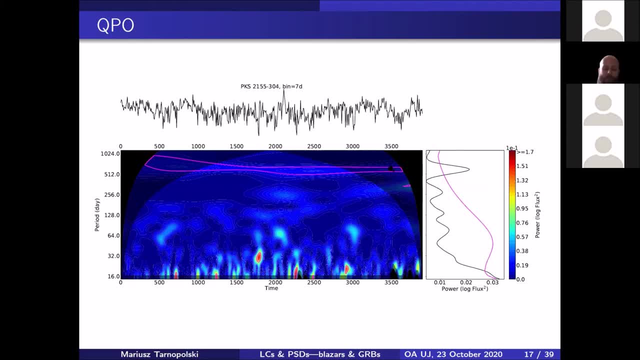 in the leading period, And this is the only QPO out of the eight reported for the objects in our sample that we detected in the wavelength on this compelling 3-sigma significance In case of the gravitational lens, this PKS 1830,. 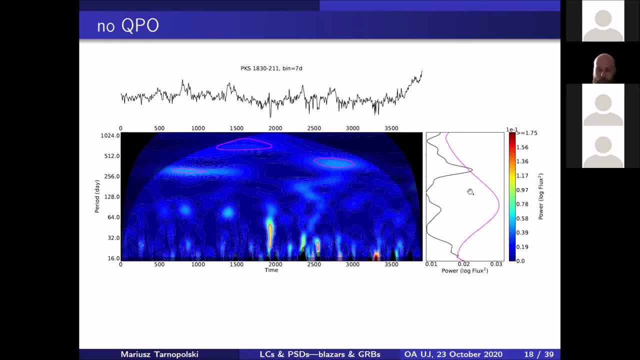 one can at first think there's a new QPO because there's this peak here. But a closer look at the escalogram shows that these lone, isolated 3-sigma contours cannot be confidently described as a QPO. They all correspond to different leading periods. 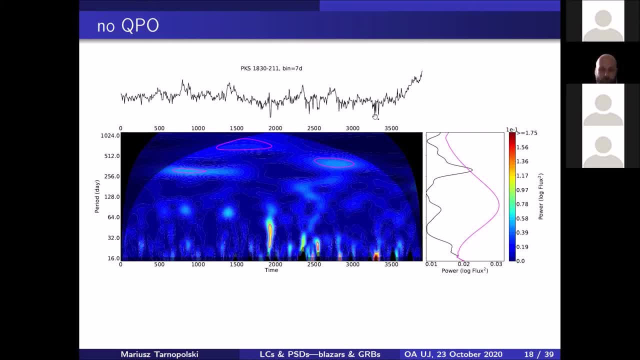 are separated in time and the features corresponding in the light curves do not show enough persistence. So, based on the global periodogram, this one on the right one would conclude there's a peak above 3-sigma, but the escalogram doesn't support. 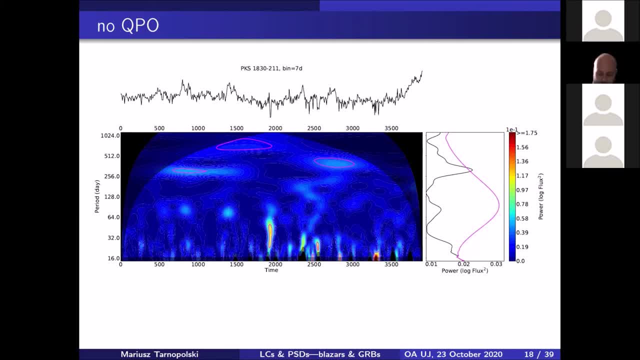 it being a real QPO. And recently, the importance of utilizing various methods for accessing the PSDs, compared with the stochalogram analysis and a visual inspection of the light curves in question, was also pointed out. So, fortunately, vigorous use of wavelets is being advocated. 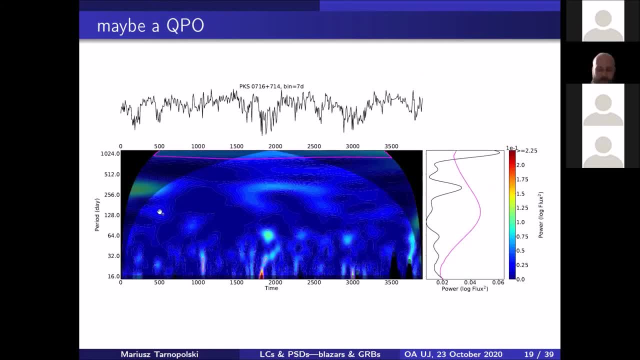 We also observed hints of a quasi-periodic modulation in another object, PKS 0716, with a much higher period exceeding 1000 days. So, given the length of the data, this definitely should be treated with caution till it's observed for a longer time. 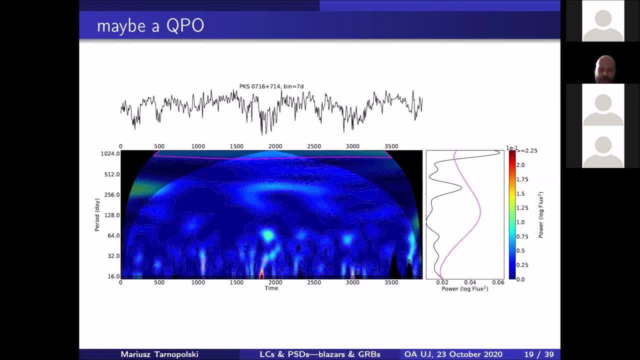 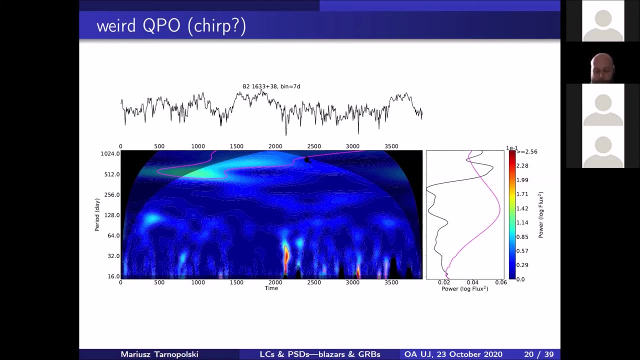 But some other authors also pointed this one out as an interesting candidate. And there was also this curious feature that looks like a chirp as the period gradient systematically increases over time. Other authors reported as well some leading periods, but those were based on an LSP approach. 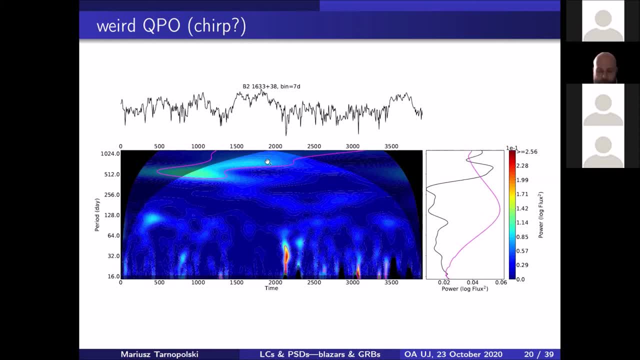 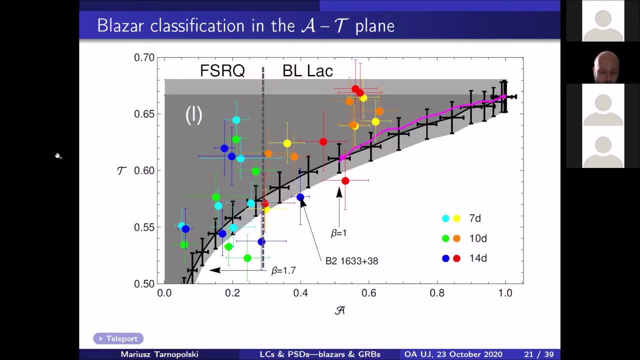 And here we see this: apparently a single feature that is evolving in time. What is actually novel and non-trivial is that the blazer types separate in the AT plane. So to give an overview, this dark grey region in the background is the region of availability. 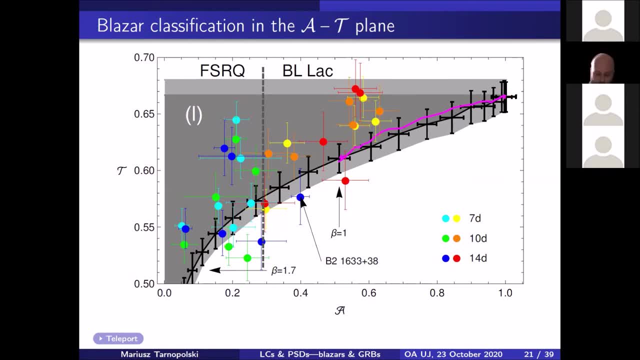 for the power law plus Poisson noise processes, With lighter grey bands around it denoting the errors corresponding to the length of the examined light curves And the cold colours of the dots denote FSRQs, while the warm colours show BLLux. 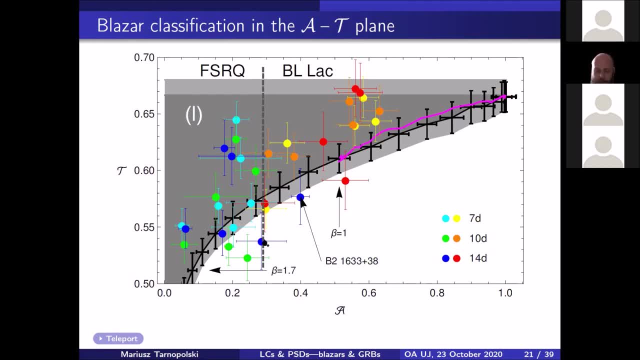 And this vertical line is the demarcation between the two, and there is this one lone outlier here. Now, this separation is not that trivial. One might say that the FSRQs have, on average, higher beta indices and are brighter than BLLux. 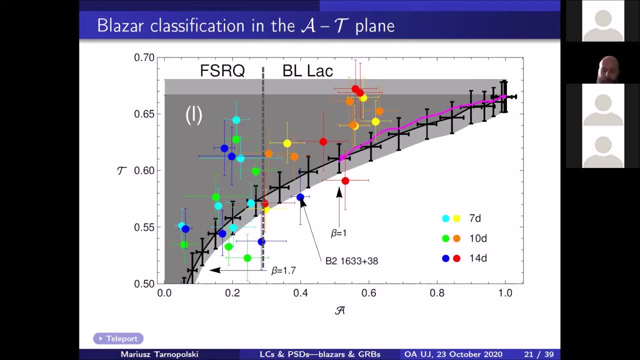 so less noisy than the observed light curves, So it should be placed on the left part of the plot. But this is not the case, since this purple line on the right shows the beta equal to one case and its path when the Poisson noise level. 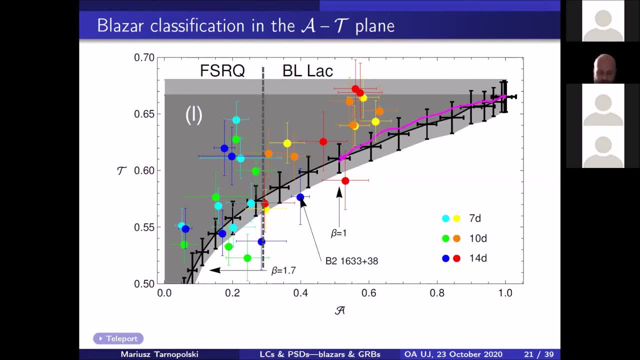 so the white noise contamination is increased. Such lines for other beta would be similar in nature, So this is not that trivial. hence the separation of blazers in the ATE plane seems to be a genuine feature, And it's supported also by our previous findings. 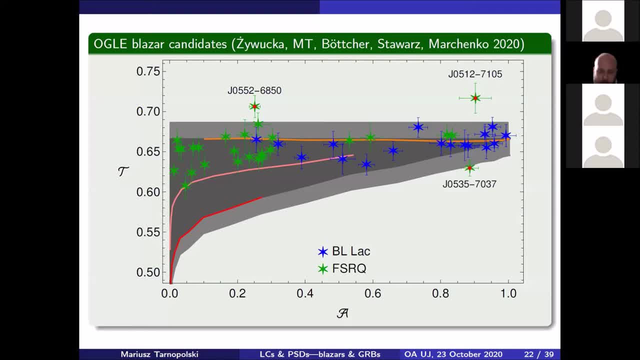 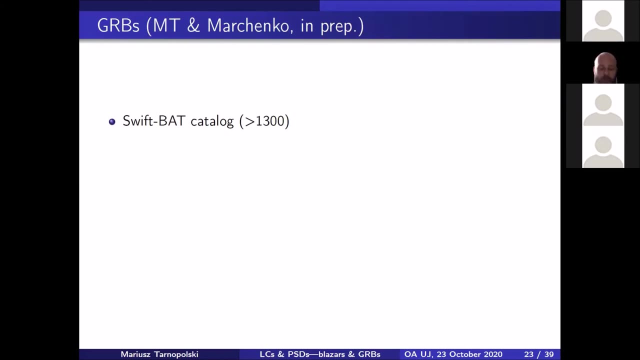 that blazer candidates behind Magellanic clouds, in the optical in this case- also occupy different parts of the ATE plane depending on their supposed classification On to the most recent preliminary results concerning gamma ray bursts utilizing the already mentioned methods. In general, we consider the SWIFT catalogue. 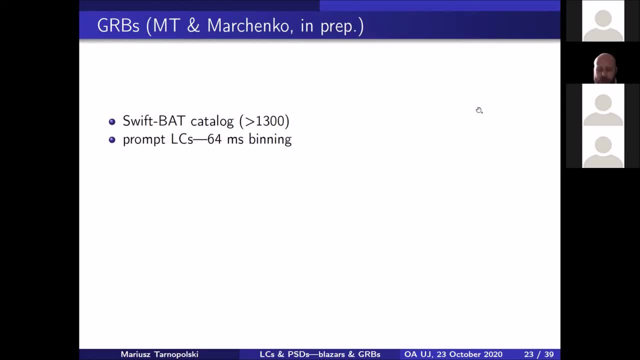 of over 1300 GRBs. We consider only prompt light curves in a 64 millisecond binning to get a uniform resolution for all of the sources. We consider only confidently long GRBs, that is, those with durations more than 3.2 seconds. 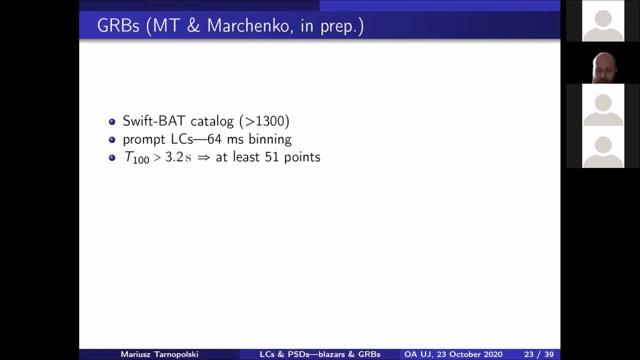 to get more than 50 points. in order to get a good sampling And to keep the sample homogeneous, we exclude confirmed short GRBs with extended emission And in the end, we end with 1160 GRBs whose PSDs were fitted with the previously mentioned models. 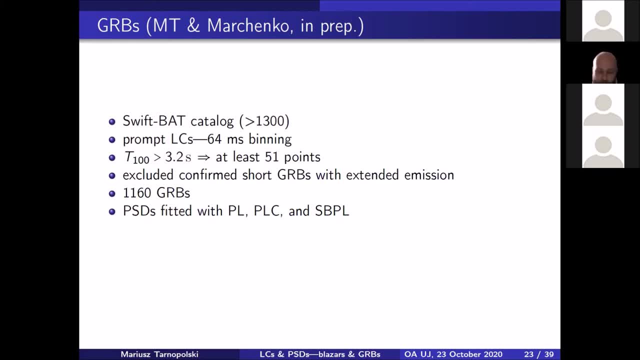 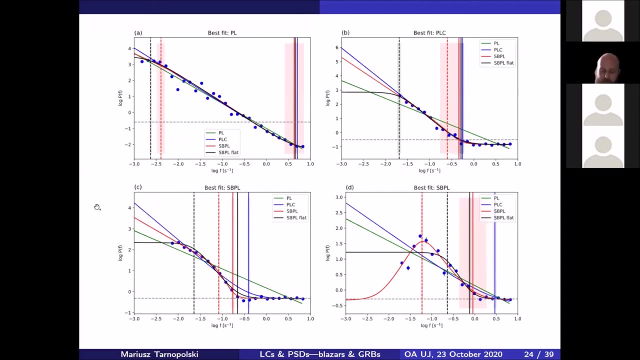 the power law. the power law plus Poisson noise and the broken power law. We attempted an ATE, plane classification and SWIFT for QPOS. So I will just go over the PSDs really fast. These are some random examples of the pure power law of the best model. 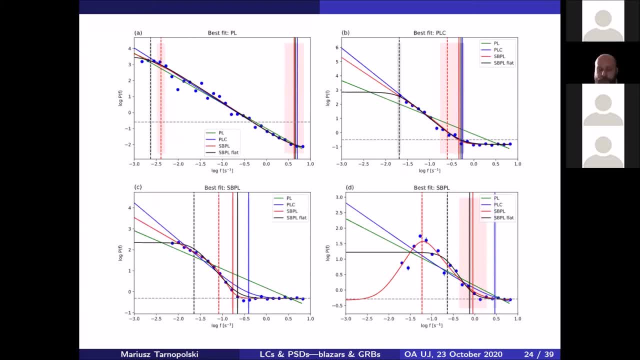 in the upper left corner, fitted to the binned PSD. Then there is this power law with Poisson noise and two instances of a smoothly broken power law. Some PSDs were quite peculiar, like this one on the bottom right that basically consists of a peak. 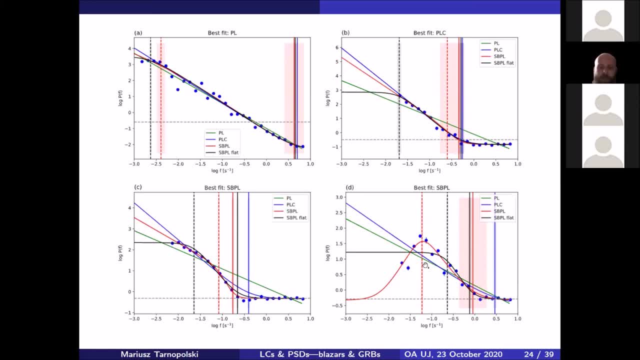 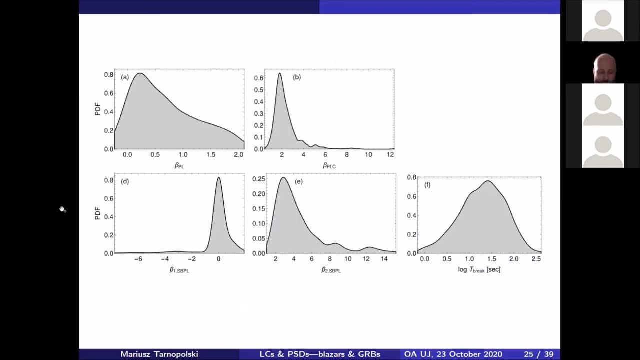 Like this whole, PSD is just one peak And in this case the small frequency index, beta1, is negative. So some descriptive statistics. The power law betas are extend to about 2.. When Poisson noise is introduced, this is between 1 and 3, mostly with a tail. 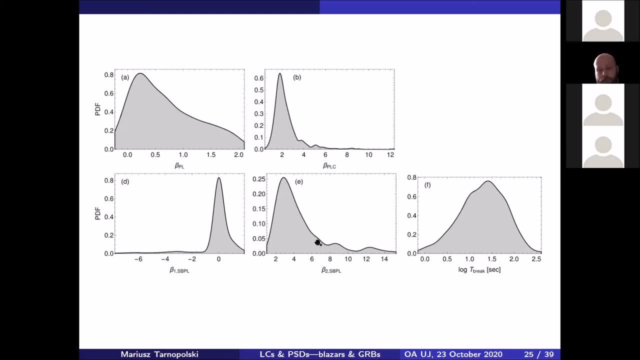 And the smoothly broken power law can be as steep as 6 with some heavier tail. And the time scales at which the break between the beta1 and beta2 occurs is roughly between 1 second and 100 seconds, with a logarithmic mean at about 30 seconds. 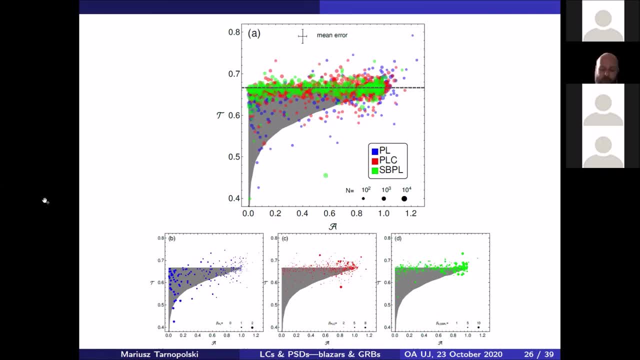 And, having these PSD types in mind, the locations in the ATE plane are surprisingly unremarkable. We anticipated getting clear clusters, but that's not the case, Although one can see some over density here around 0.123, but that's the location of white noise. 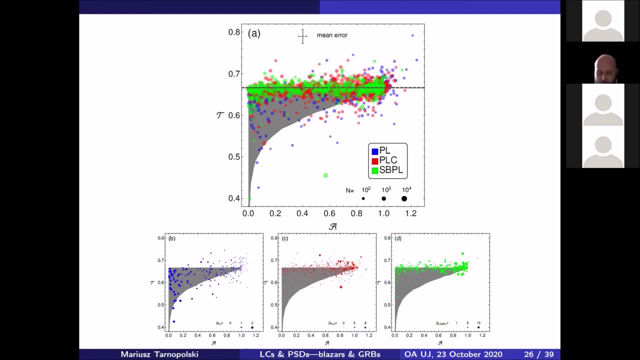 and many GRDs in the catalog are very noisy, dim and with low signal to noise ratio, And using only the high quality data doesn't reveal any substructure either, And within each PSD type the power law case behaves as expected with higher beta further to the left of the plot. 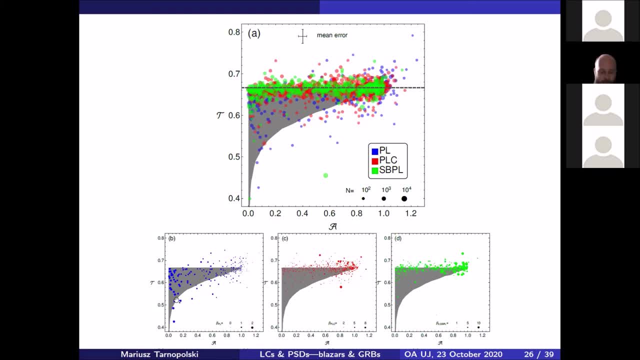 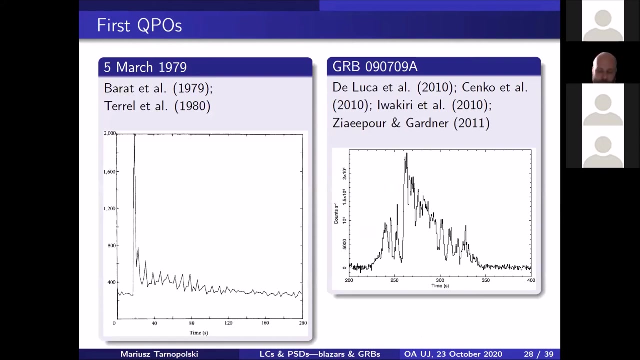 indicated by the size of the points here. But the power law, Poisson noise and broken power law behave erratic, likely due to the high noise contamination. Maybe I will skip this to save time. The first QPOs in gamma ray bursts were reported back in the 70s. 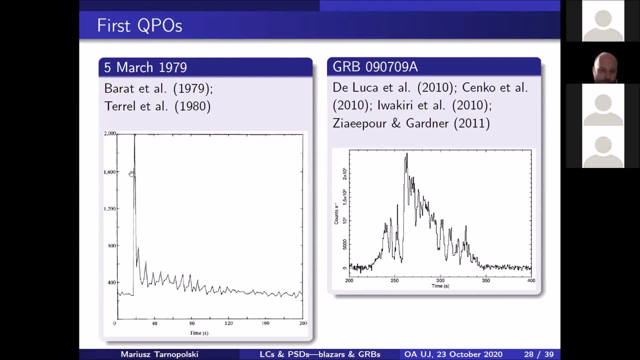 and it consisted, after the initial outburst, of a steady modulation with about an 8 second period lasting for about 20 cycles, And this is probably the highest significance QPO ever detected in a GRD. More recently, there was some interest about 10 years ago regarding some SwiftGRB. 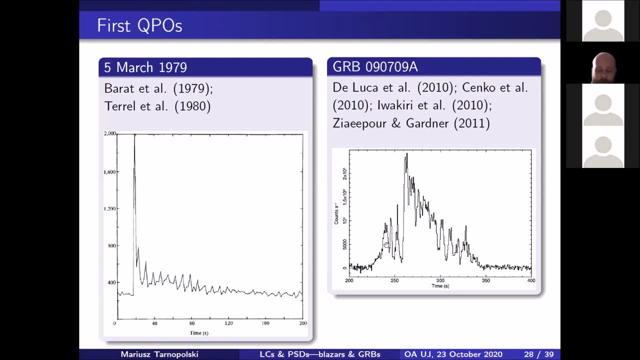 which also seemed to exhibit 8 second modulation on top of a pulse: the fast rise, exponential decay shape. There were a few works at that time utilizing data from different spacecrafts like Integral, Suzaku and so on, but they were yielding very, very varied results regarding the significance. 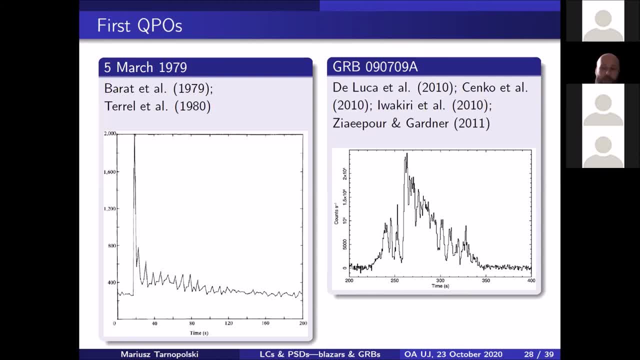 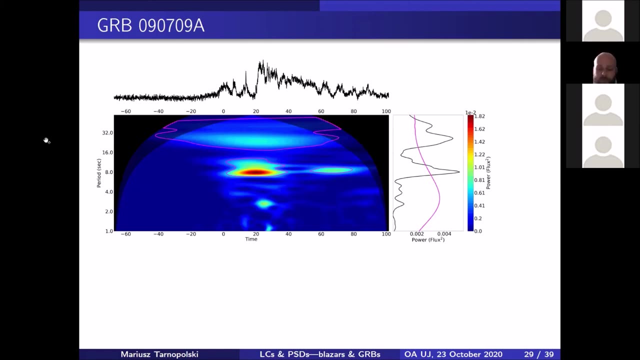 even for data from the same instrument but analyzed with a bit differently by different groups. So this is the first GRB whose collogram I will show. I mean, this is this event from the 10 years ago And we see here quite a constant. 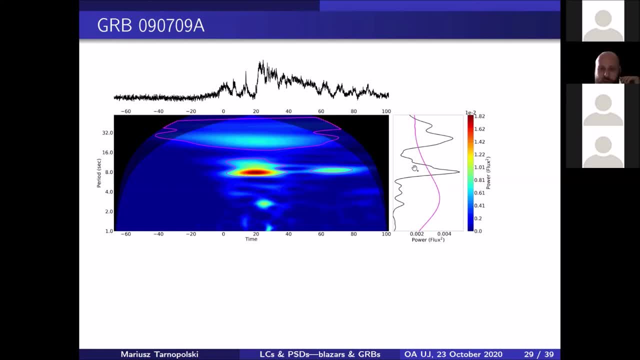 and persistent modulation that they reported about 8 second period. So it's 8 seconds lasting for 80 seconds. so it's more or less 10 cycles. Now, just for illustration, I will be showing a few sinusoidal fits to the time series that were done. 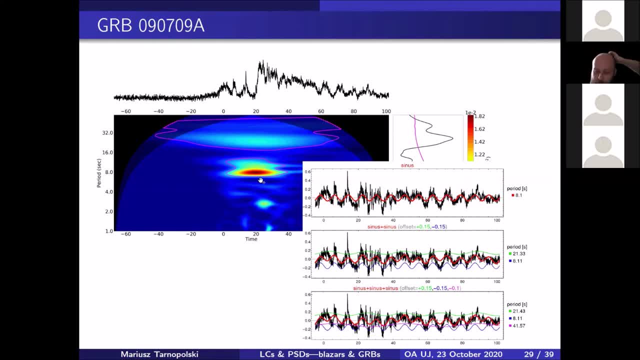 using the periods identified from the scologram. But I like to stress that this is purely for demonstration here, just to guide the eye, to visualize the character of the modulation. This is not that we are fitting a sign and claiming a QPO. So the 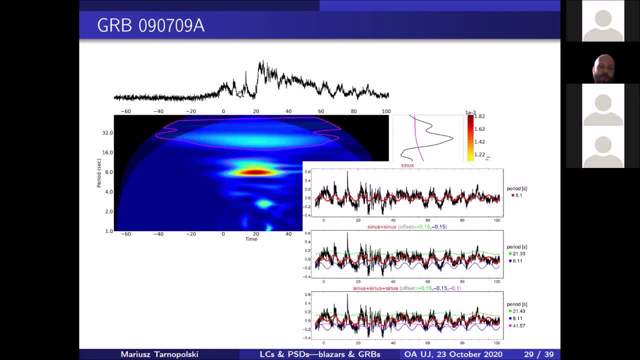 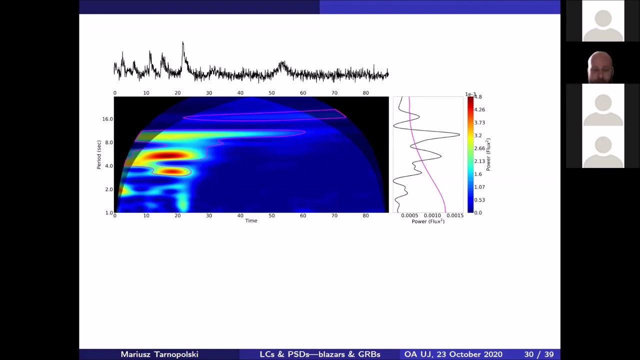 And this cycle here is slightly different than the one on top here, because first I fitted and removed this pulse and the wavelet scologram. the implementation that we utilized takes care of the trending by carefully fitting a polynomial. Okay, So a few plots and that will be almost it. 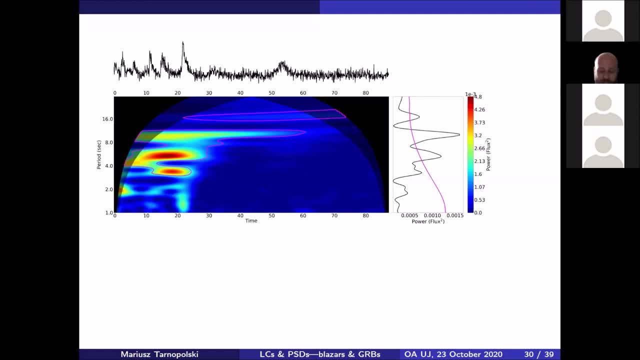 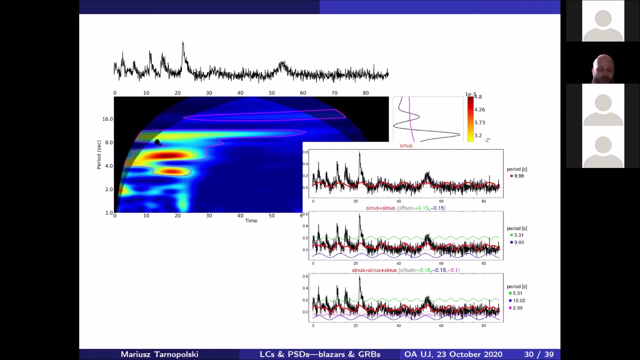 Here is a series of apparent harmonics, maybe with an overall increasing period, which manifests in the light curves as systematically growing. separation between and the sinusoidal fits are not good here, since each of these pulses is non-sinusoidal and so describing the whole light curve. 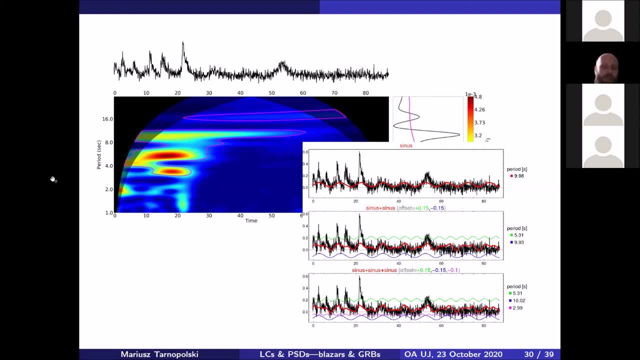 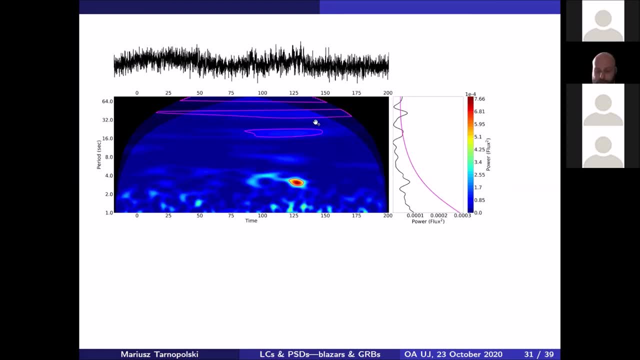 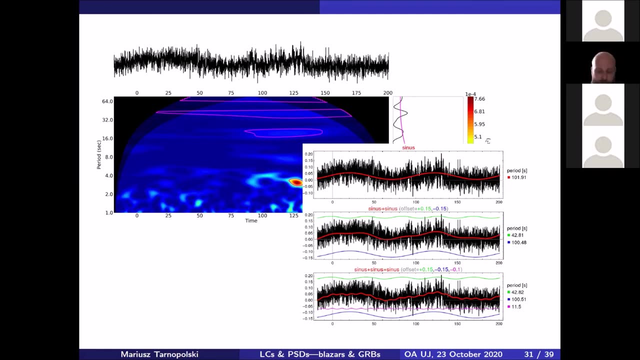 as a combination of signs is not appropriate. So in this case there is this 40 second modulation, But actually the first sign that is identified is about the 100 period and it's just exceeding the range of the period shown in the scologram here. 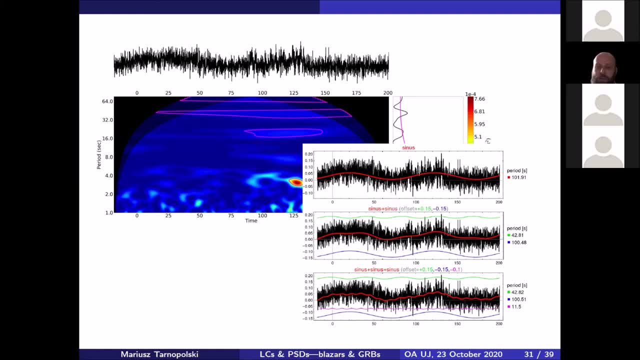 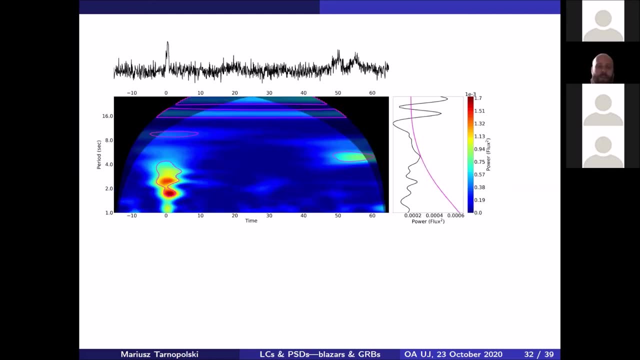 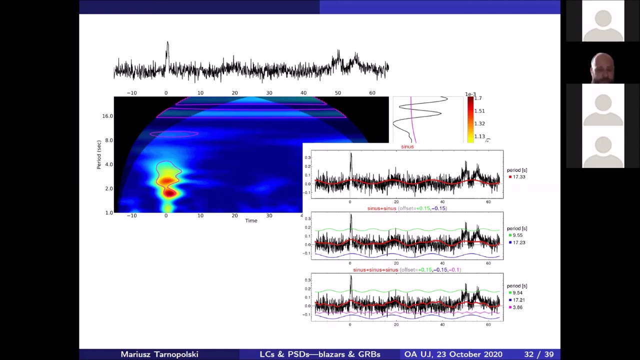 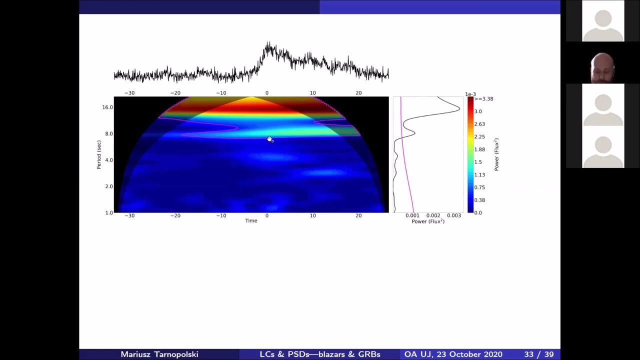 But on top of it there is again a 40 second period roughly consistent with this identified QPO here. Here is a similar feature with a 17 second QPO, neatly in this case visible as an approximation of a sign, And another example with basically two main modes. 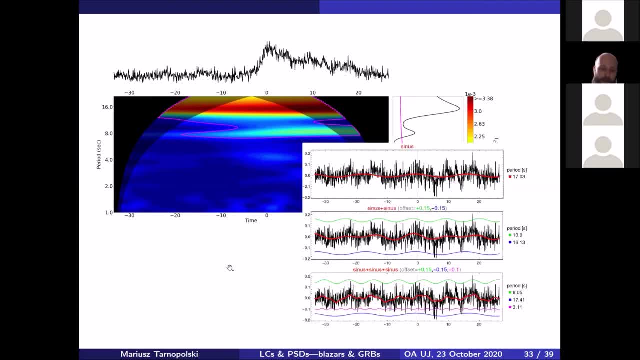 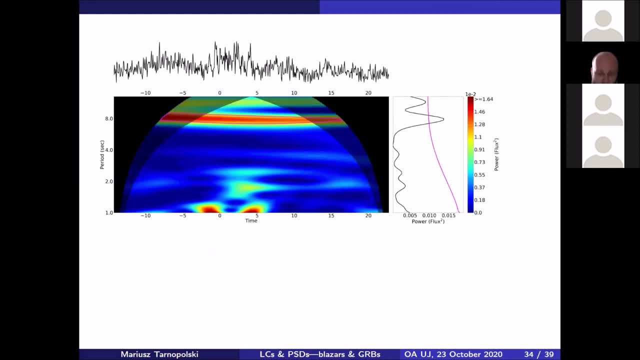 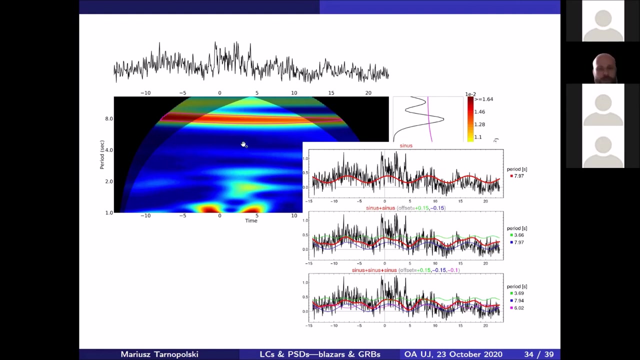 Again on top of a pulse that was, for the sake of this illustration, removed, And this is the probably most pleasant case of a very clear 8 second QPO lasting for about 4 cycles, And this also quite nicely fits the sinusoidal scheme, and this is like the only prominent feature. 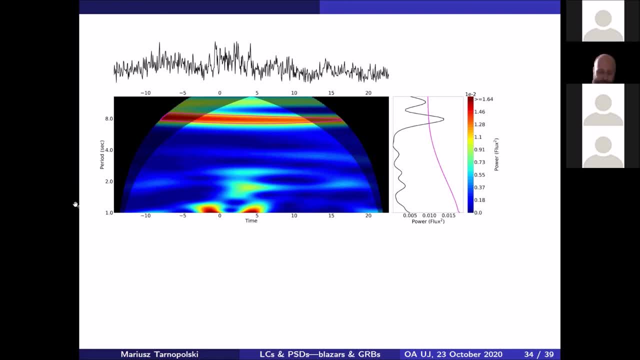 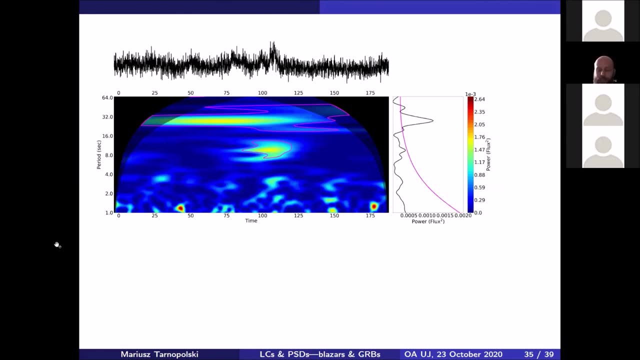 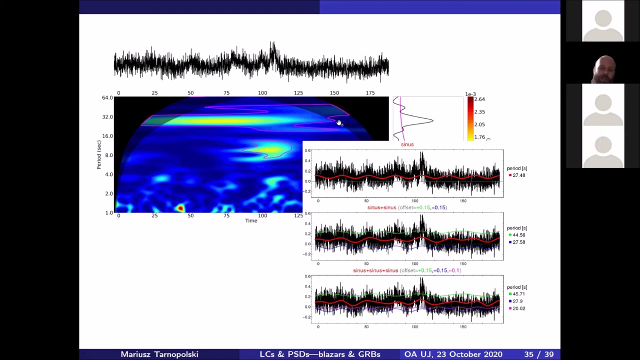 in the whole scologram. But this best illustrates that additional signs, sign waves, may actually ruin the fit, because it may lie well on some portions of the fit and fail for some others, Because the modulations that are present here last only in parts of the light curve. 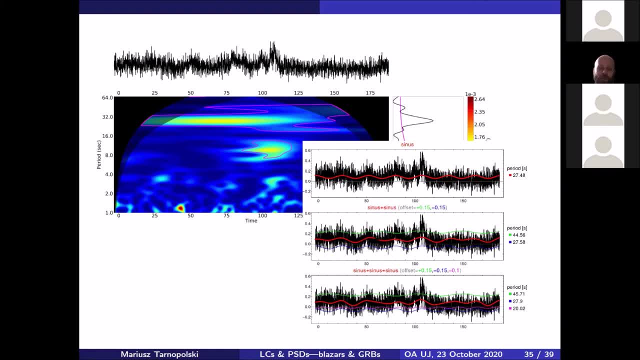 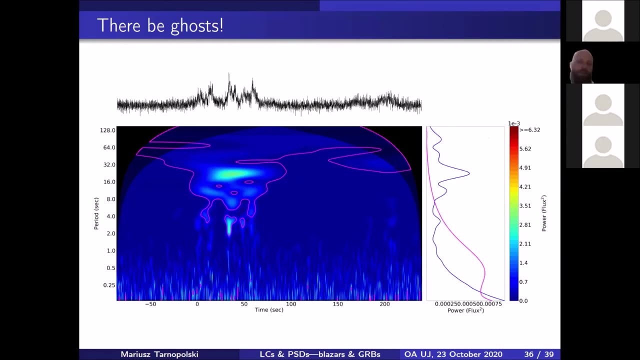 and the signs are fitted globally to the whole light curve, even to the parts where the modulation doesn't exist. And there is also a bunch of complicated, much more complicated than the ones that I just showed- features difficult to interpret, All looking kind of like an extraterrestrial ghost. 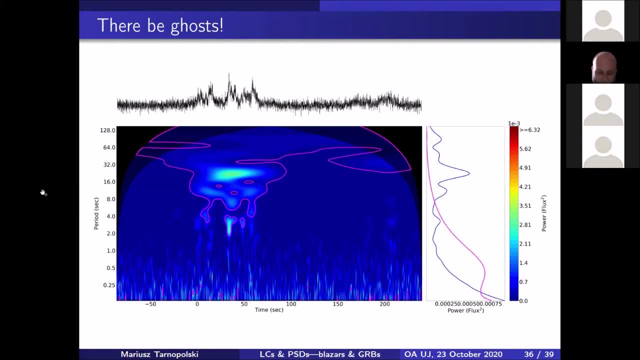 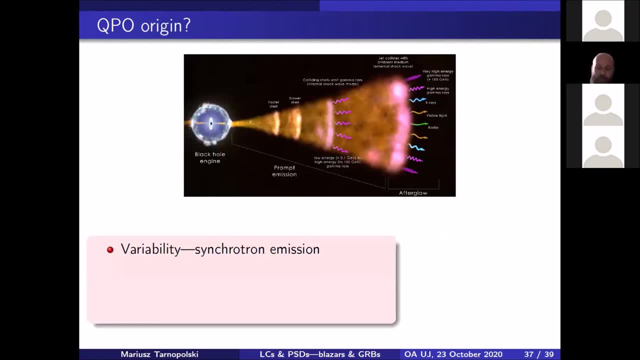 lurking at us from the deep space. So the unanswered question is: what causes these presumed QPO's in GRBs? In general, the prompt emission is of synchrotron nature and comes from colliding shells within a relativistic jet powered by accretion of a remnant material. 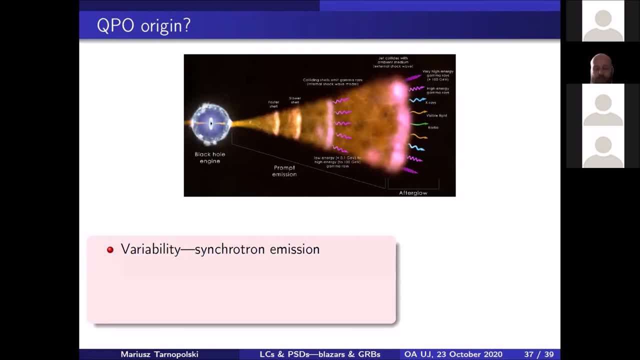 There is one worked out physical scenario pertaining to short GRBs, but we analyzed only- confidently- long ones, so it's unclear whether the same mechanism applies or not, And some other from the top of the head interpretations might be that these QPO's are due to some mechanical modulation. 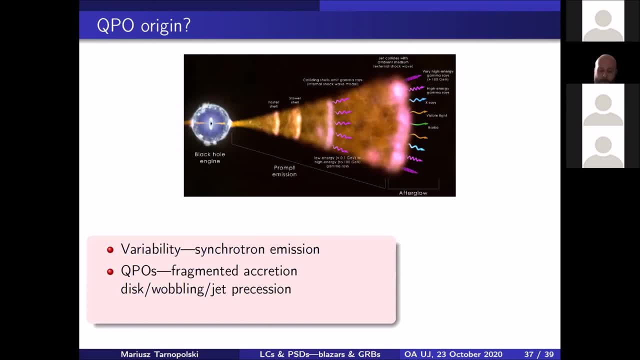 in the disk or jet, while the origins, while the origin of chirps, if real, is even more mysterious but might be caused by emission during fallback of remnant matter from a fragmented disk in spiral link on trajectories inside the innermost stable circular orbit. So this has an 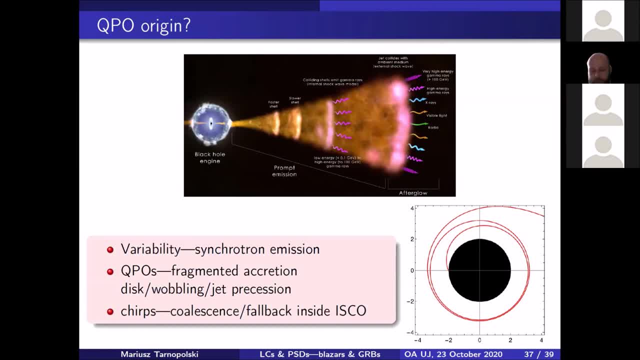 has a decreasing period. that might be manifested as a chirping signal in the light curve. This needs to be calculated more precisely, that is, the time scales, the required masses and so on. So basically, the governing mechanism is unclear. so there is definitely place for future explorations.